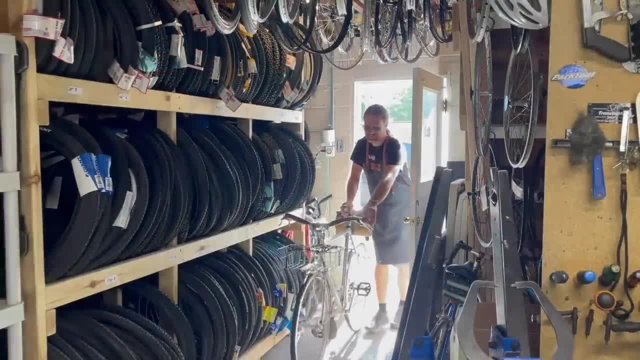 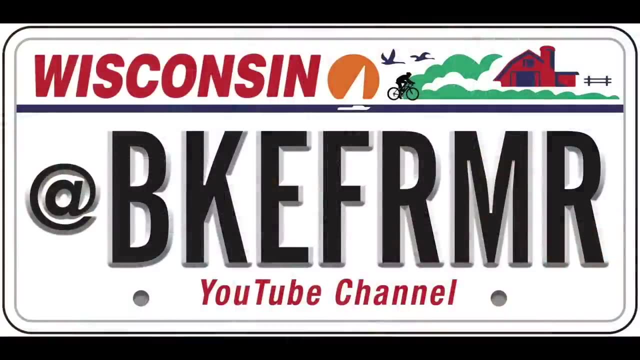 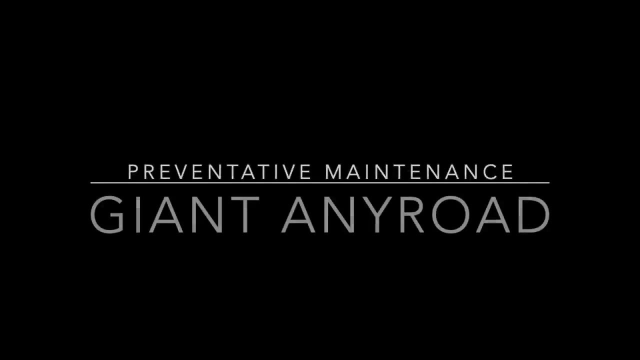 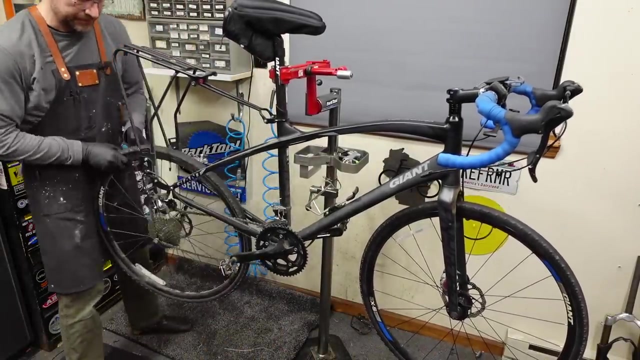 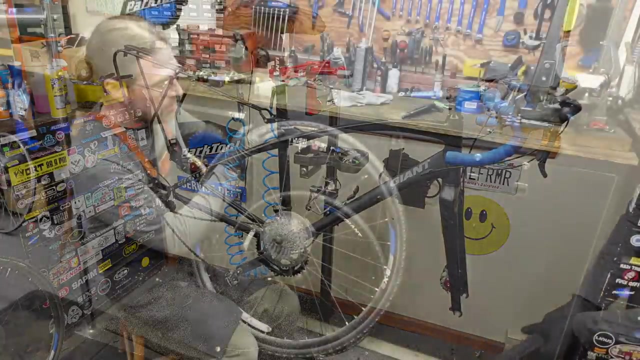 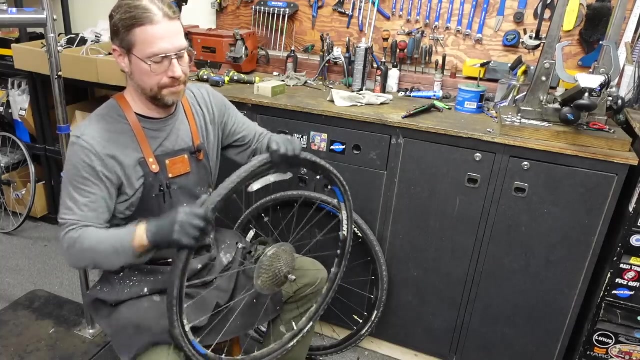 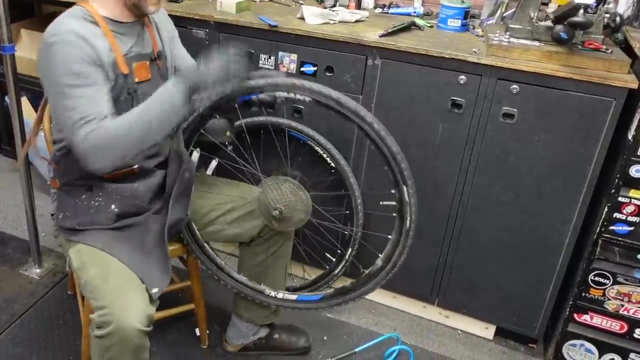 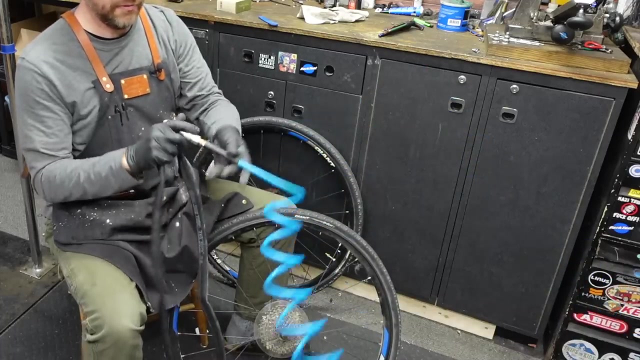 here we go. Okay, per the usual, first thing I'm going to do is pop these wheels off. So, like I mentioned in the intro, it's got a flat tire. I'm just going to take care of that right away. Okay, let's put some air in here and see if we can find the hole, figure out what's going on. 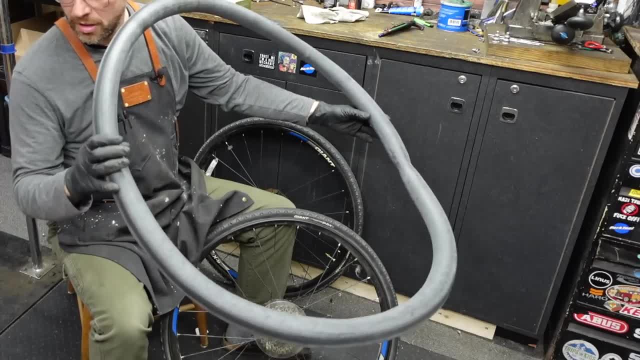 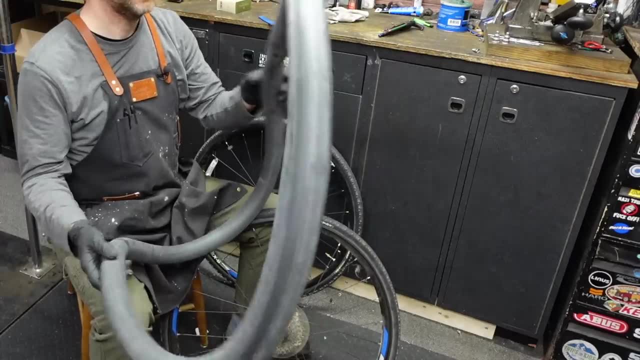 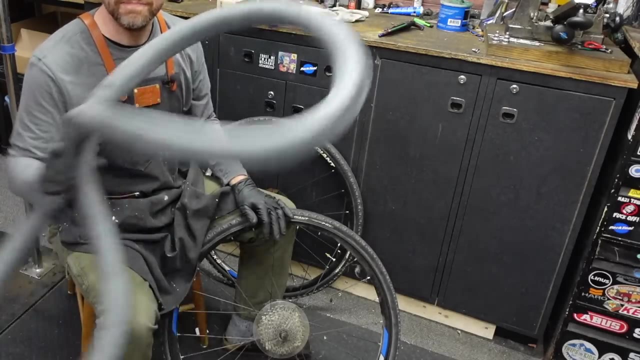 Well, it's nothing obvious In cases like this. I just assume there's a tiny hole in the tube. somehow. It was flat as a pancake, so we'll put a new one in. I'm going to go through and see if I can find something sharp, Slice my finger open. 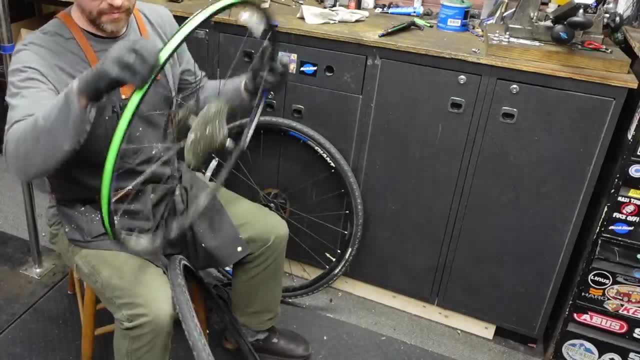 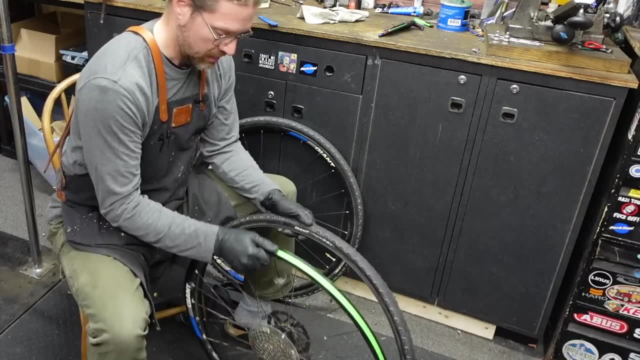 I'm a risk taker, Check the rim same way. I figure it'll cut my rubber glove and I'm just going to say bad luck is what caused that flat. We don't always find the reason and it sure ain't worth fretting about. 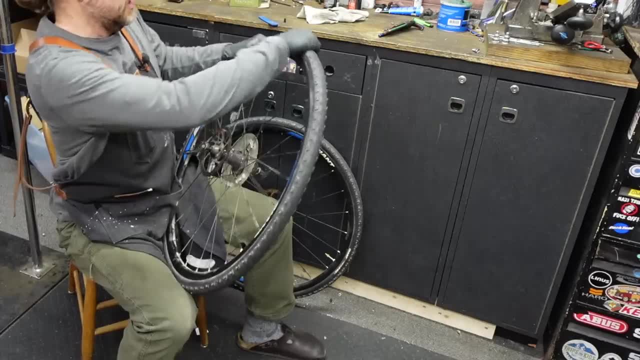 So I fill it up halfway, and then I'm going to go ahead and put it back in. Okay, so I'm going to go ahead and put it back in, And then I'm going to go ahead and put it back in, And then I kind of go around and seat it. 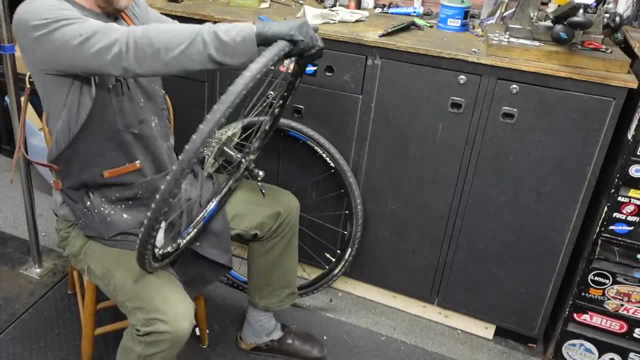 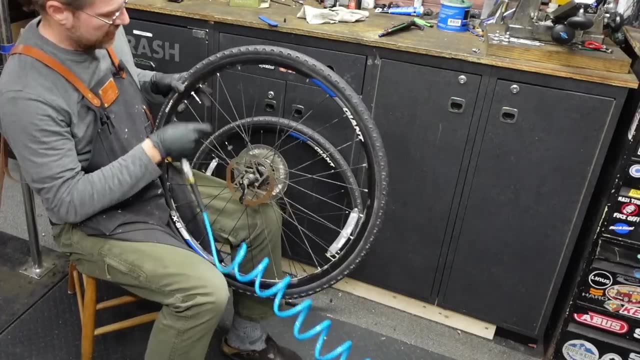 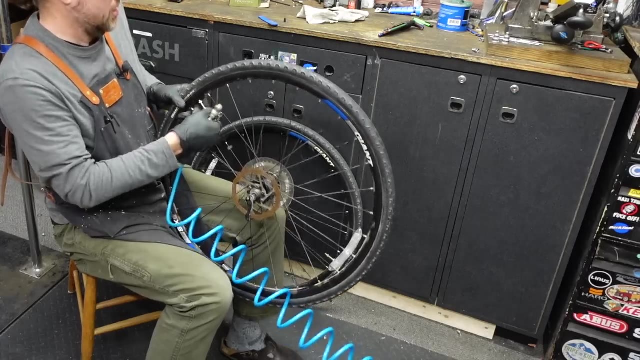 This is just a good practice: to go halfway and then just check your bead all the way around and try to get it nice and even before you cram a bunch of air in there. Way less risk of blowing something up. I'm just putting a ton of air in there. 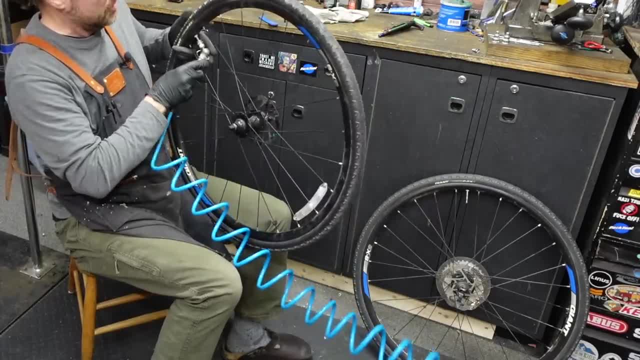 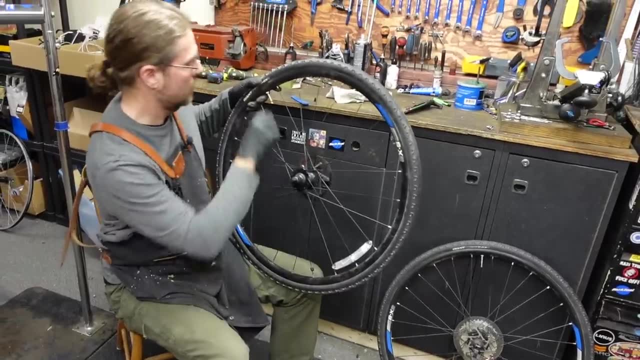 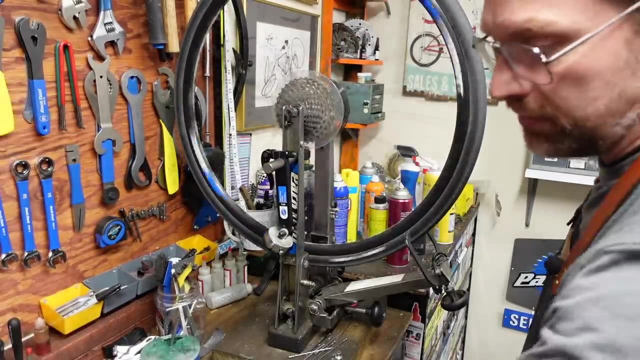 Okay, Air up this other one. One, two, All right. Tires are all good. Let's throw them up in the truing stand. Now, this isn't something I'd expect you to have at home as a do-it-yourselfer. 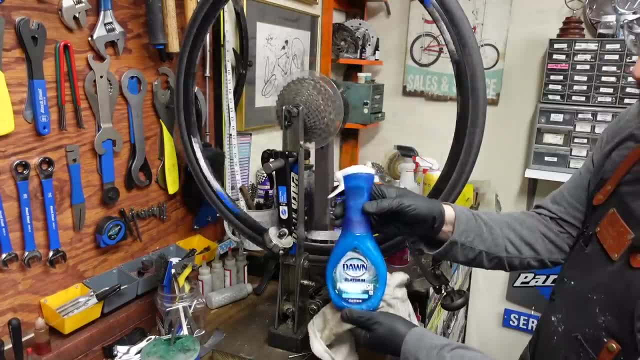 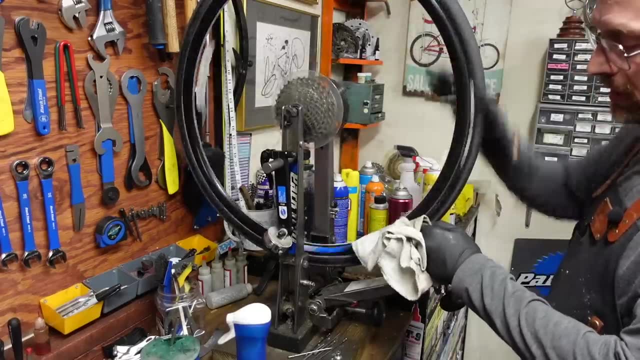 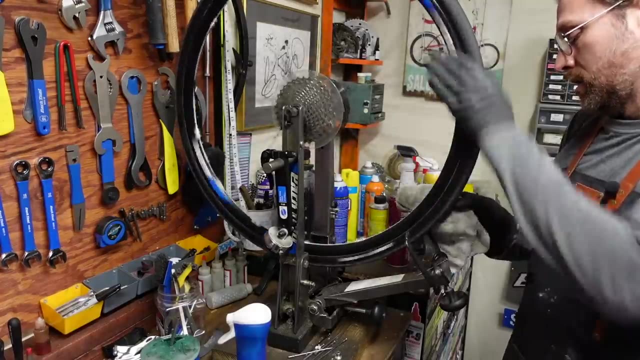 but you can do this while the wheel is in the bike too. I'm just going to take a little Dawn Power Wash, Squirt things down. That's a really nice cleaner Kind of clean the side of the rim, Clean the other side of the rim. 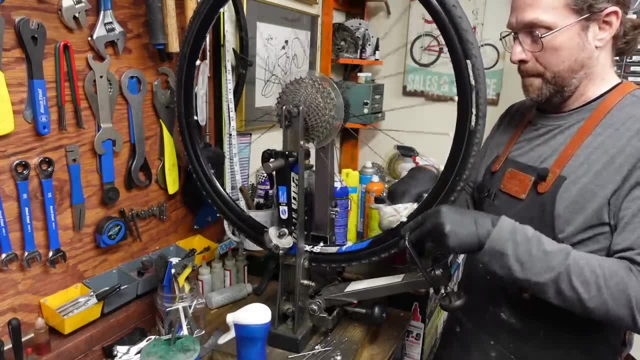 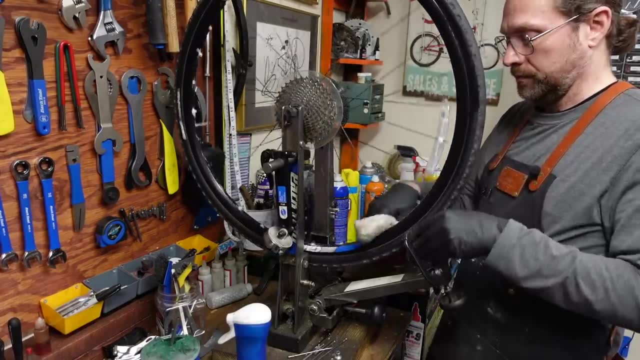 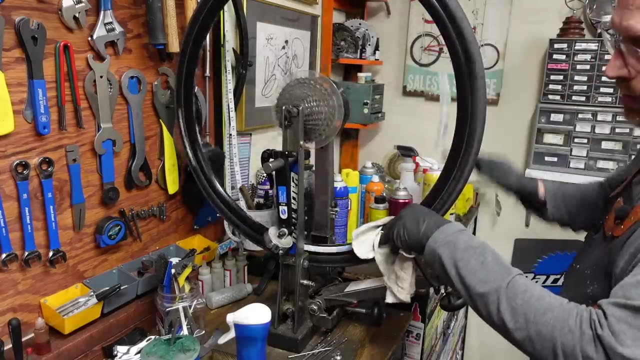 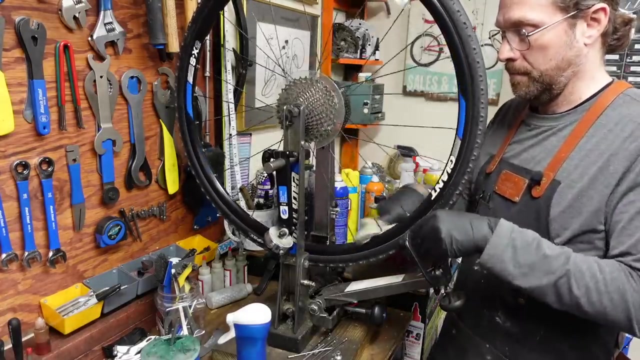 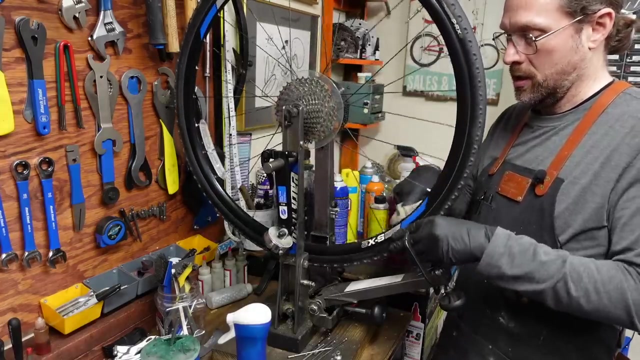 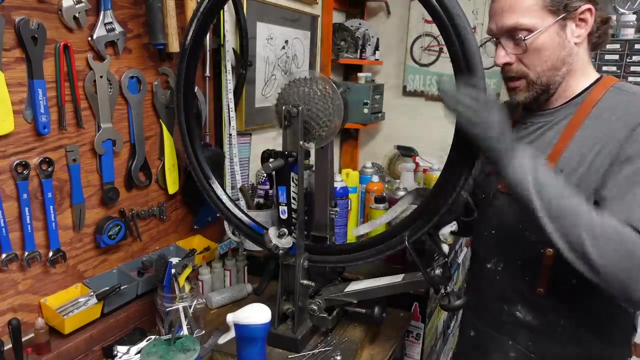 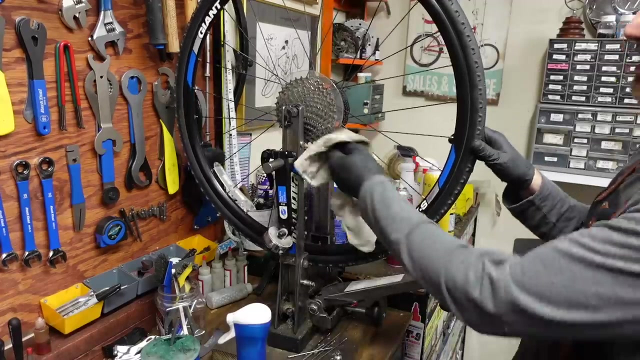 And then I go through and I floss between the spokes, Wipe up a little of the excess, Go through and do it again, Get it to that stage and I go through and the rag has a nice tack to it. It kind of almost becomes a tack cloth. 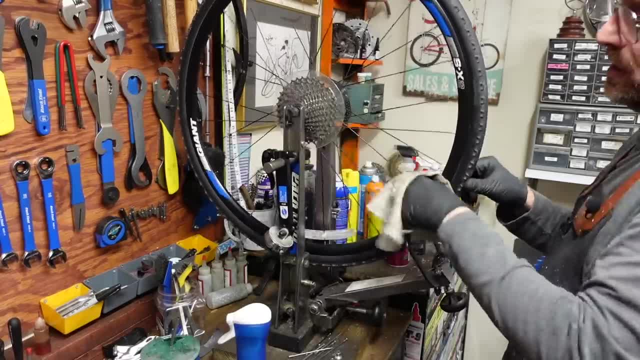 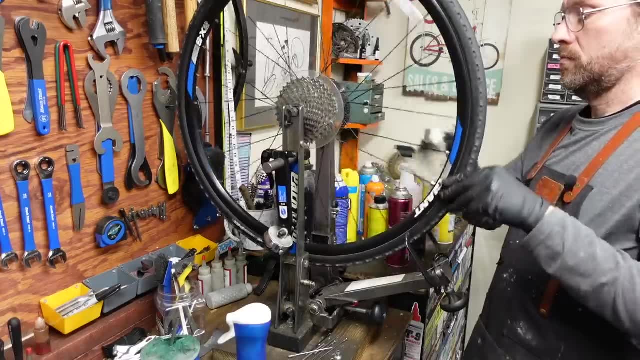 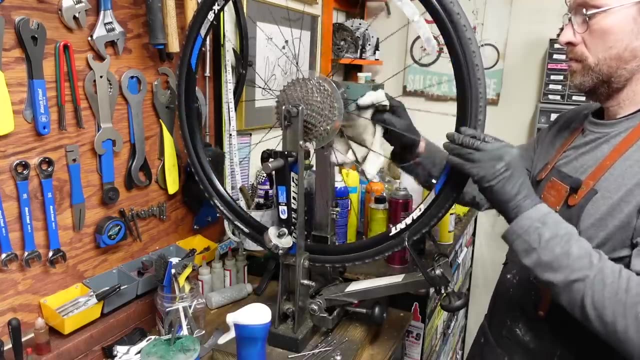 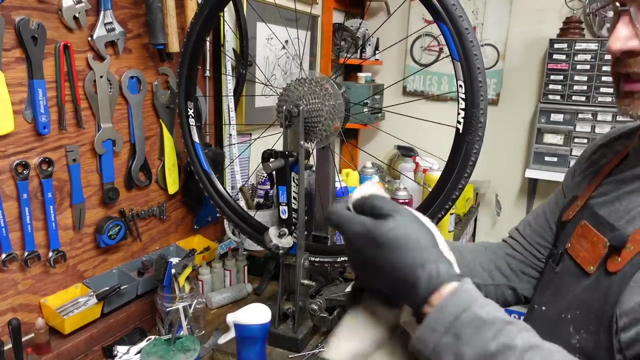 You can go through and wipe down each one of the spokes. Just get the grime off of them, Okay. And like I said, by this time your rag is nice and damp. You can just get a finger in and get back and polish the hub. 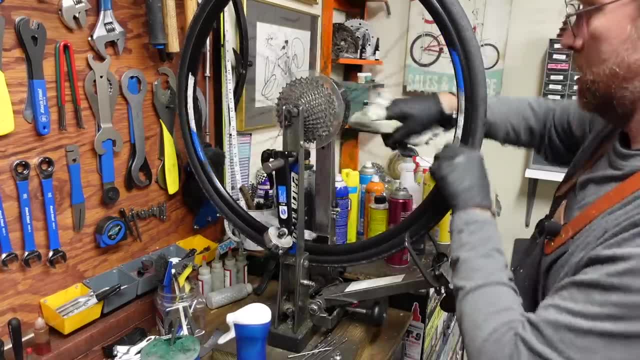 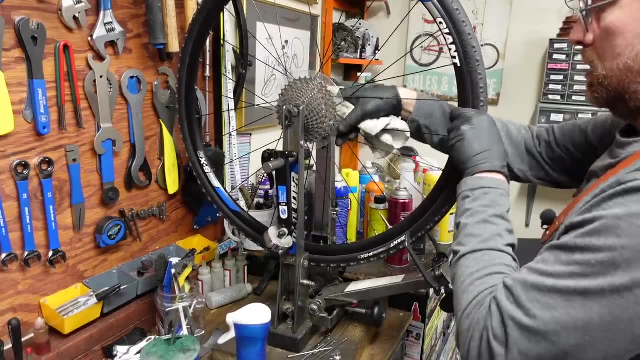 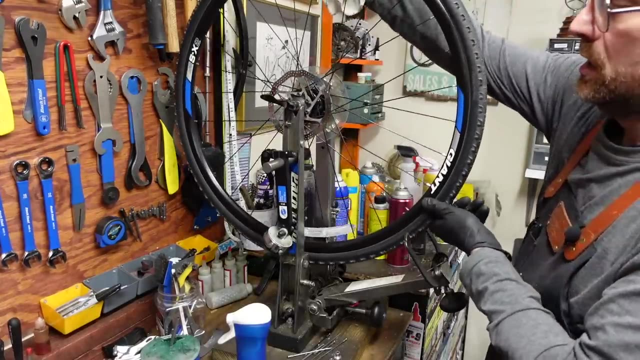 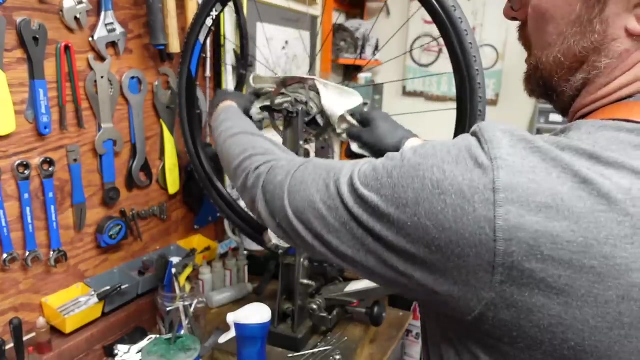 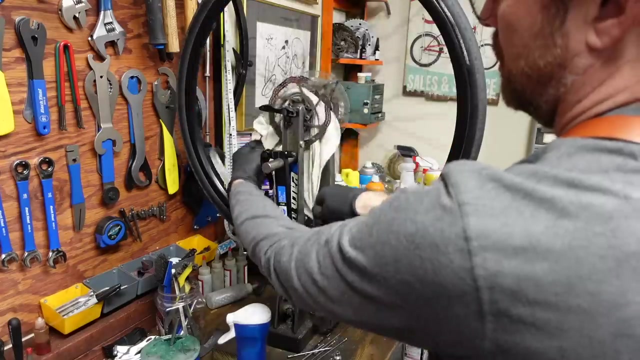 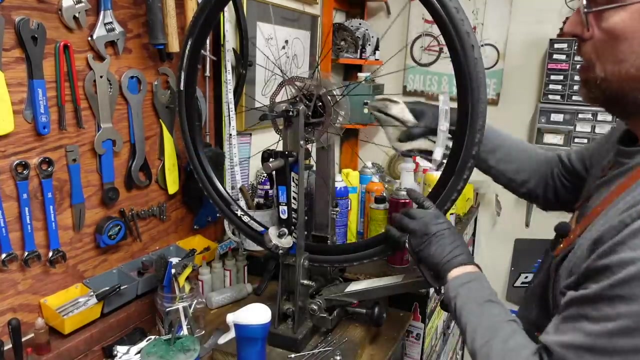 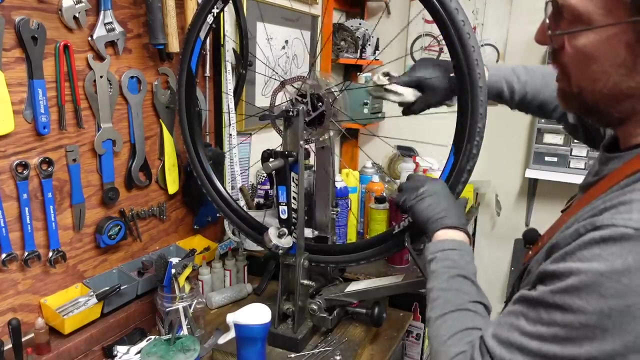 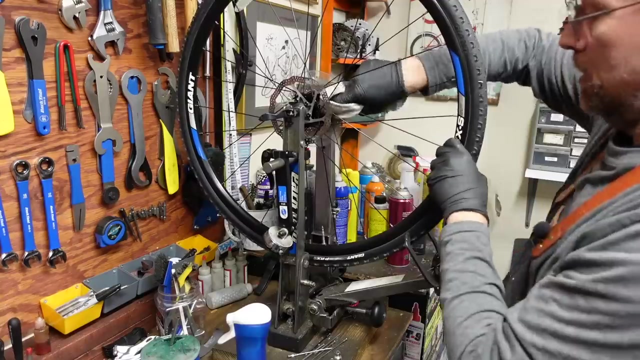 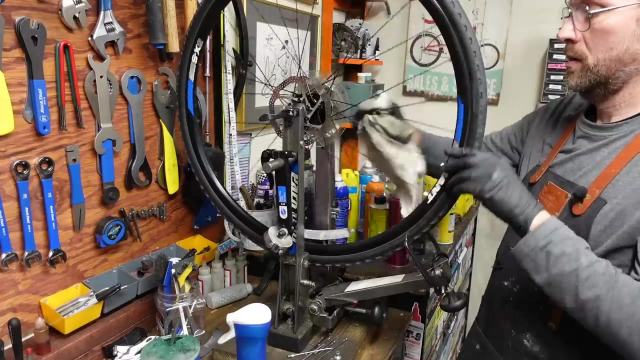 And of course when we have a disc brake we don't want to get chemicals on the disc, On the actual braking surface, So you can just kind of work the rag around Getting a finger in there again on this hub Going over the spokes again. 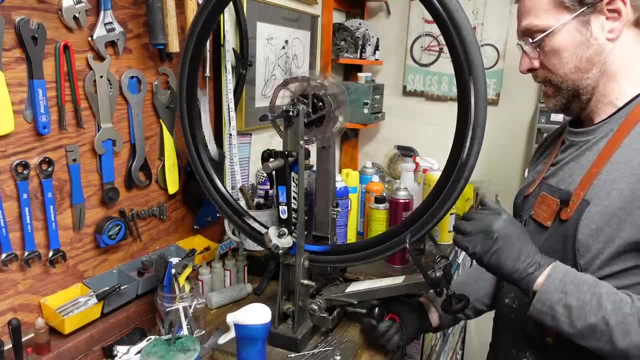 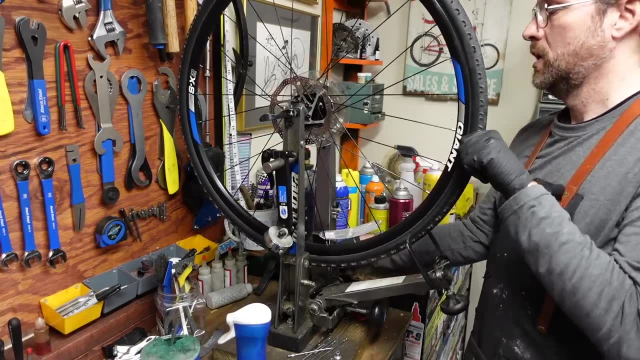 And then, since I know what I'm doing And I've got the truing stand And it's not a big deal- I always check the wheel for true And this one's like super straight, So I'm not even going to touch it. 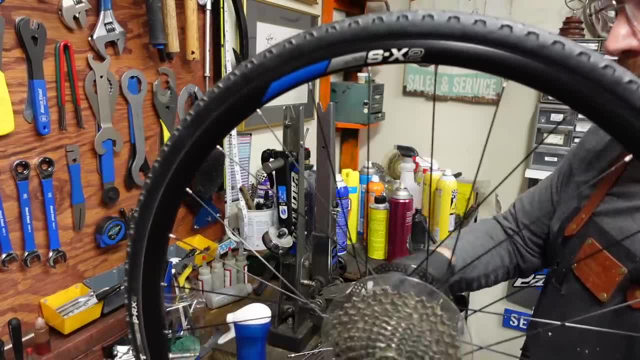 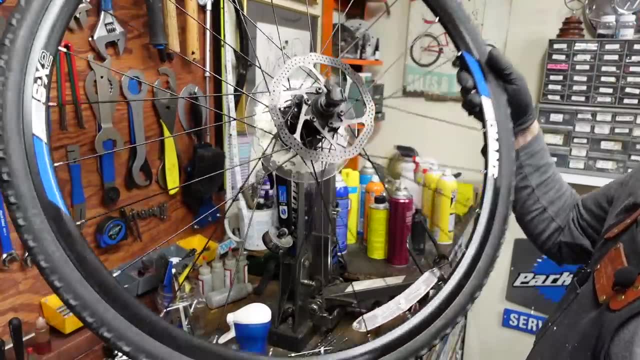 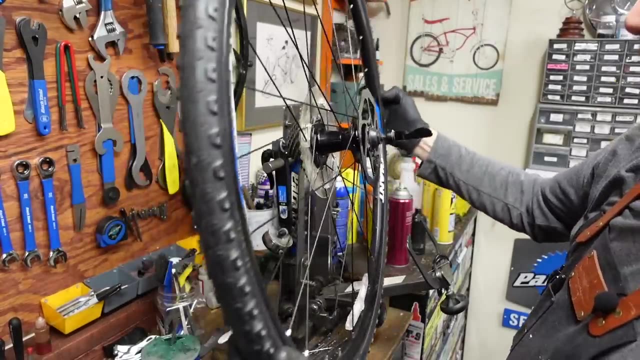 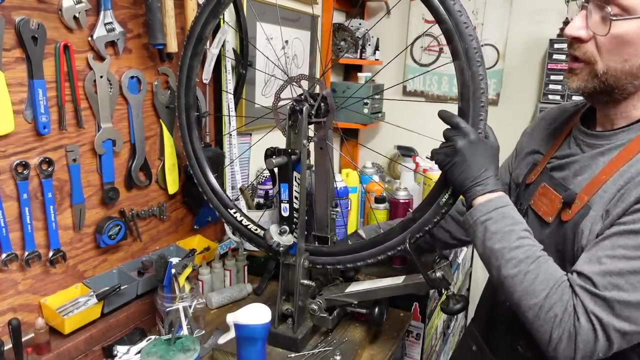 Feel the hub. And again, with hubs, I don't touch them unless I feel a reason to. So that's all good, You can see how clean it got, And then we're going to repeat that whole entire process For the front wheel. 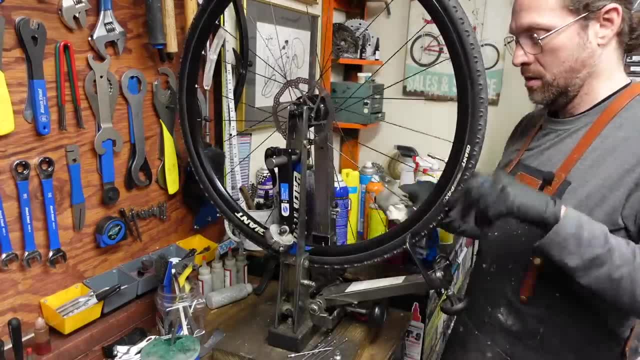 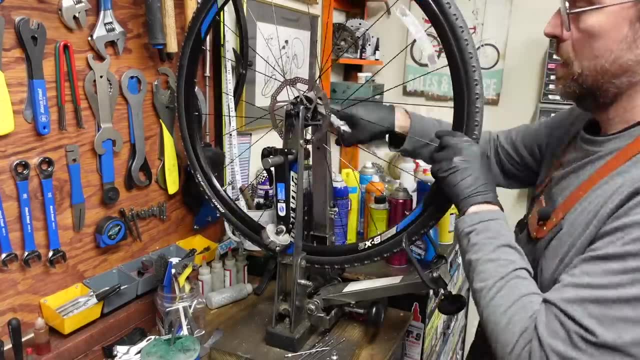 I'm just going to lay the hub back on the ground And then you can bang it in. Then we put it back on the ground So you can see more anteater. grease on it Just a little bit, Almost one. subụán. 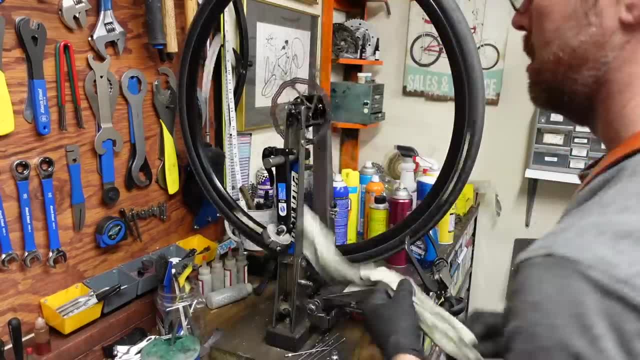 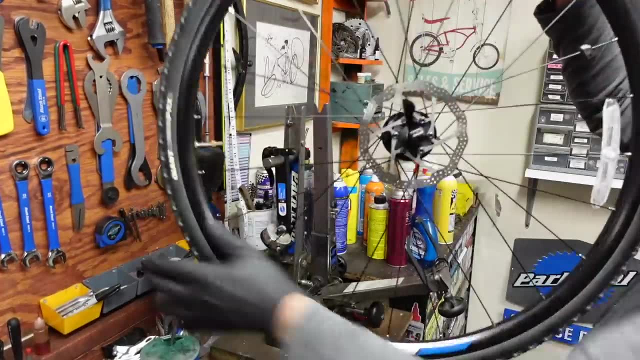 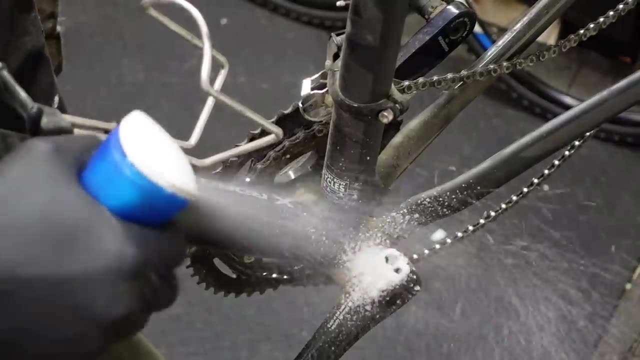 But, as you can see, I've pretty much tlined it. It will always come off, Yeah. yeah, We've got an awful lot of brush work to do, Just to have a go. So you can see how dirty this bike got. 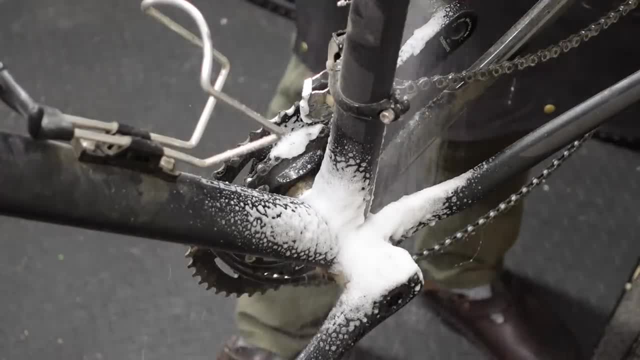 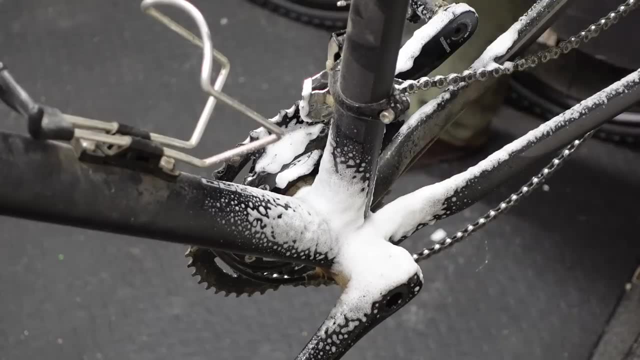 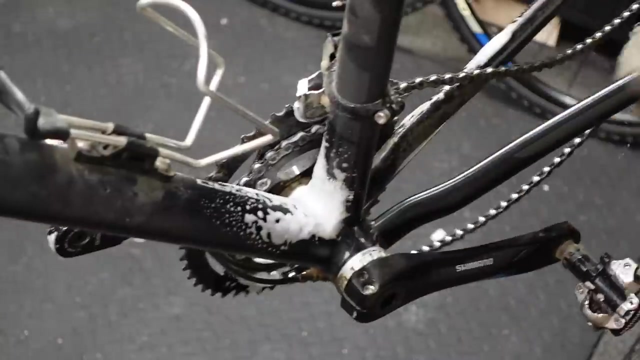 Yeah, And I think he was mainly using it for crushed limestone gravel, bike trail kind of stuff. So that's quite a bit of power wash. You really don't need that much. But it was so dirty And I'm using a kind of dirty rag here too. 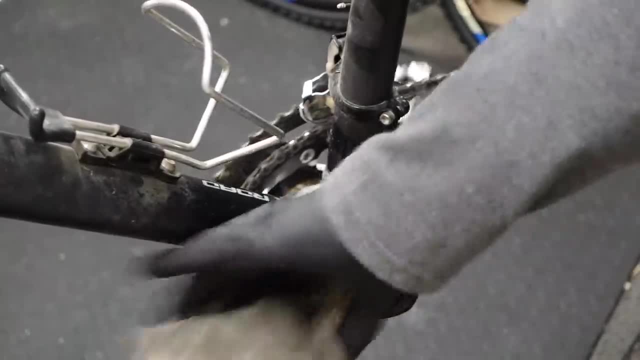 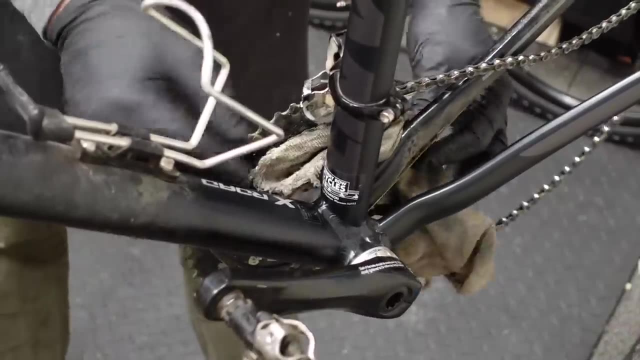 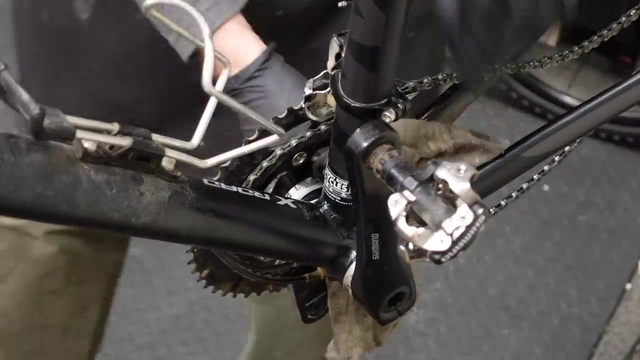 No sense in using a clean rag when things are this filthy. I just used good, old-fashioned elbow grease. The floss technique is really good when you're dealing with the nether regions here. If you've never flossed your nether regions, you're really missing out. 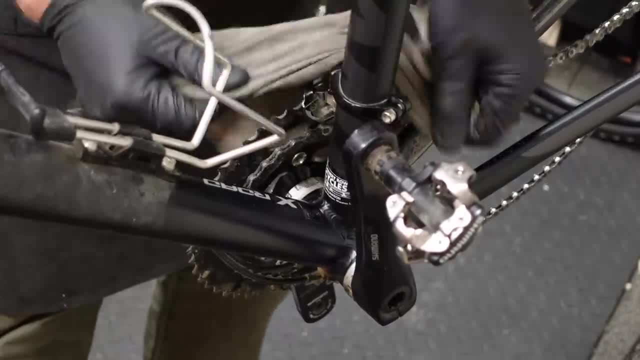 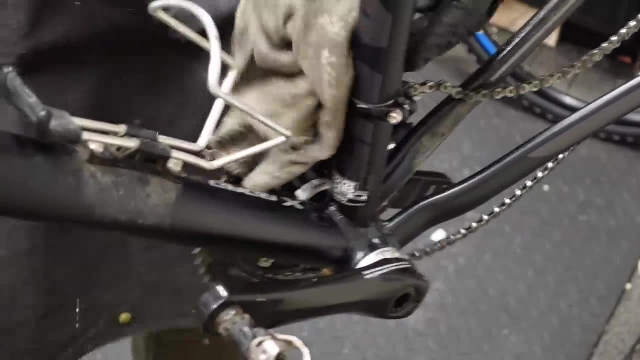 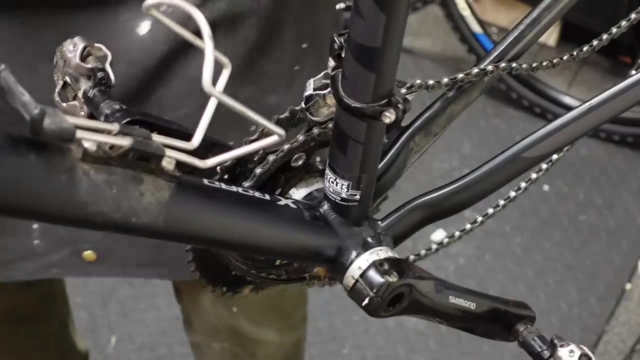 You know, it's okay to hit your bike with a nice garden hose too, But here in Wisconsin, in the middle of winter, it's not always possible, And then everything's got to dry too, But I just wipe everything down. This is just more of the same. 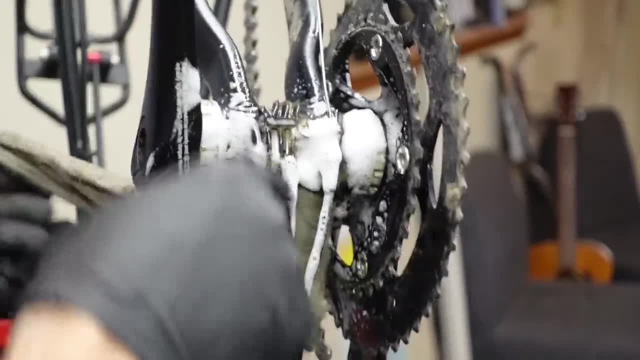 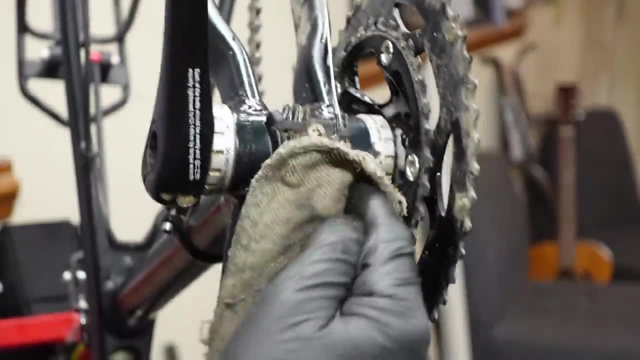 And I don't always go into this much detail when I'm doing a regular tune-up service. But this one is really pretty dirty And there's not a whole lot more that we're doing to this bike, So I'm just going to give it a little extra effort here. 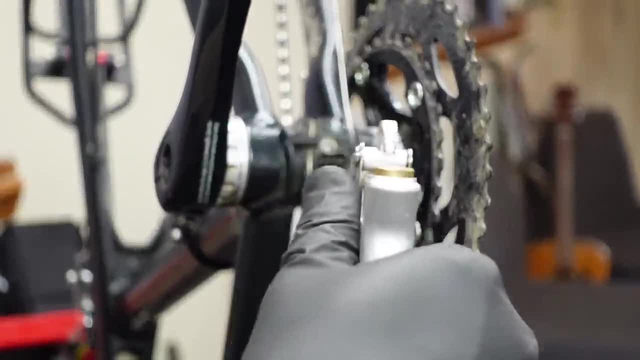 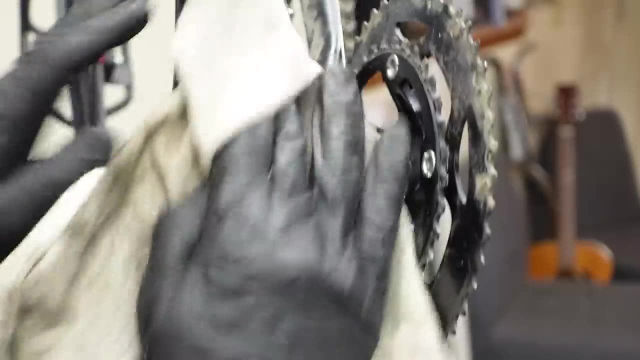 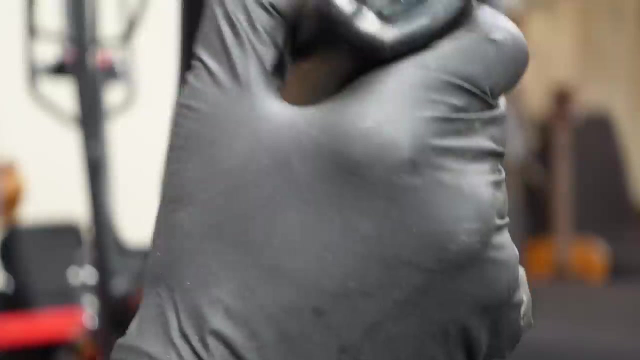 If you have access to compressed air, it's a good way to get in all the nooks and crannies, And then, while I have the bike upside down and I have access to these cables, I might as well lubricate things a little bit. 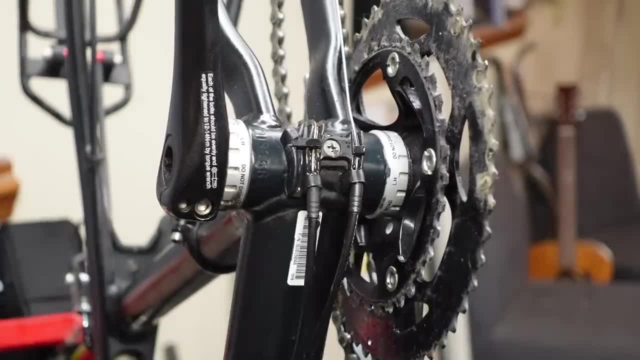 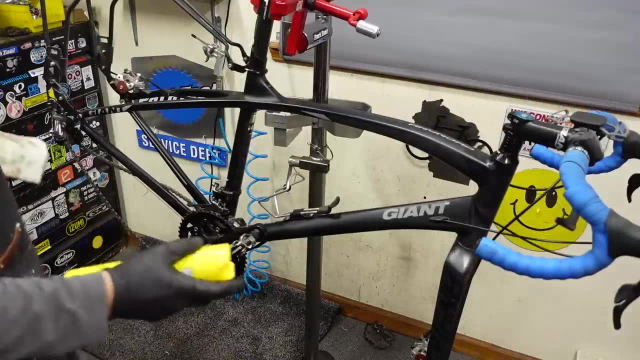 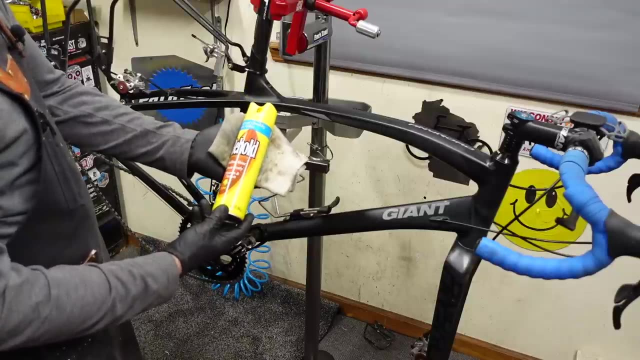 I can let gravity kind of suck that lube down into the cables. I don't like to touch cables on internally routed bikes unless I have to Once you have the bulk of it knocked off. my favorite bicycle polish is I think Behold might be taking the lead here at my favorite. 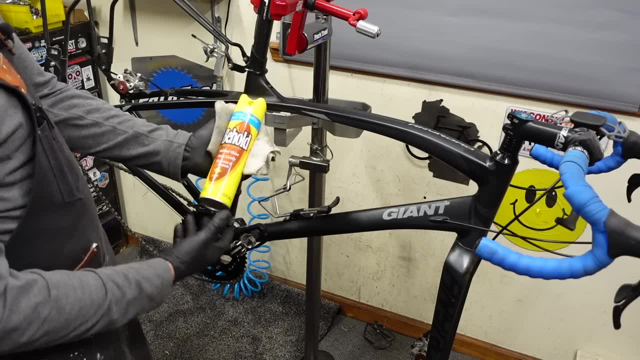 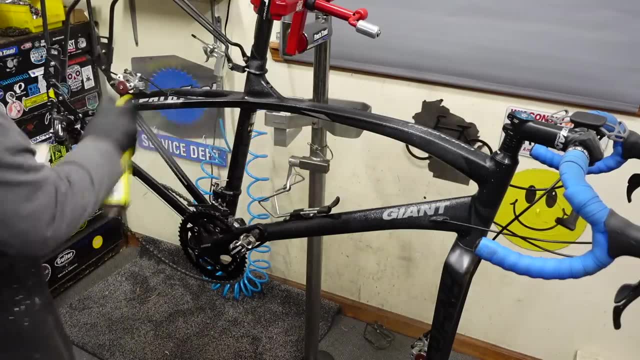 But any Lemony Fresh Wooden Furniture, Polish. I like the cheapest stuff you can get from the grocery store Which happened to be Behold last time, And it really works well And you can just kind of spray everything, Everything but your discs. 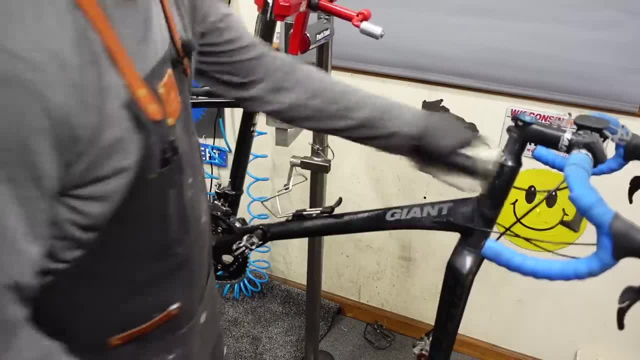 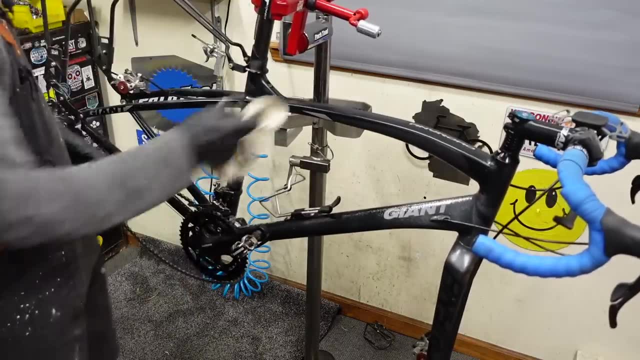 And your pads. I mean I guess I just took a little bit of a risk there with the disc brake pads, but Not too much of a risk. But that really shines a bike up Like new. It's the best trick in my book. 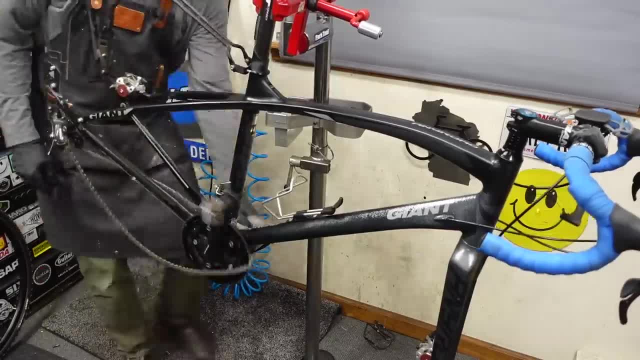 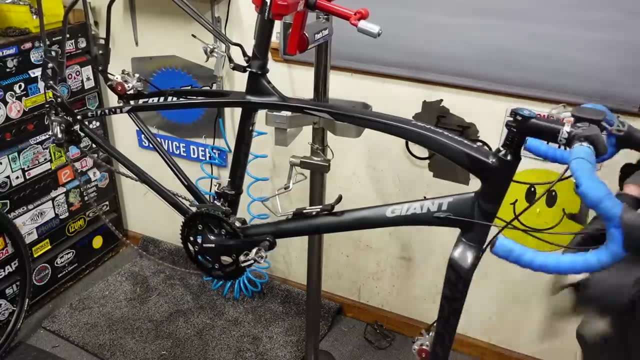 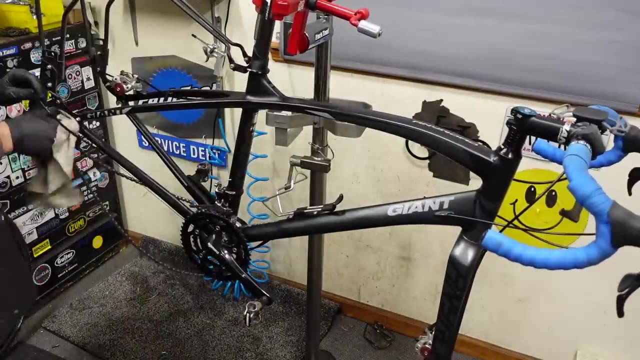 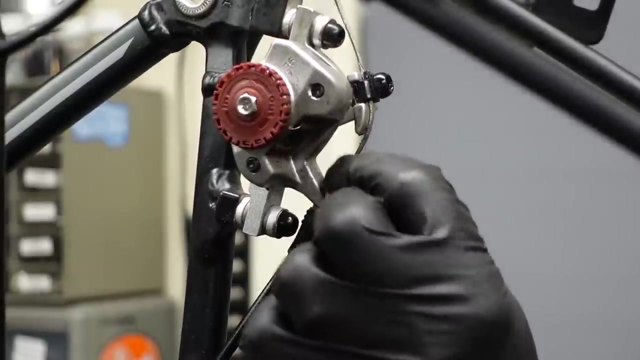 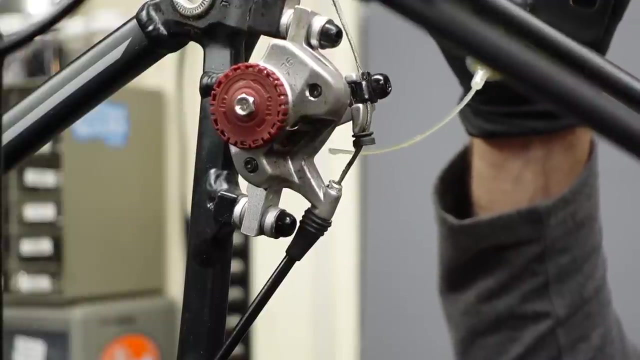 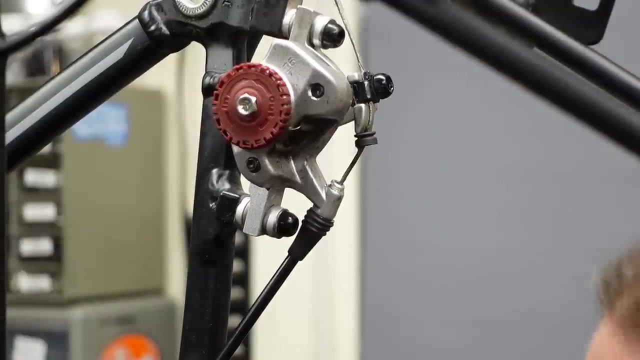 No need to buy anything expensive, Like I mentioned before, when you have internally routed cables. I don't like to take cables out of the bike, It's just inviting trouble. It's not always a big deal, But You can let gravity do a lot of the work. 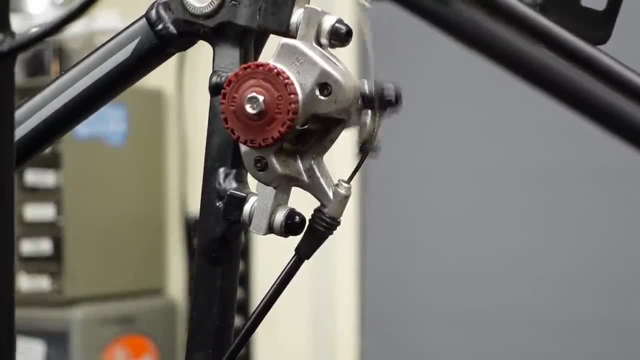 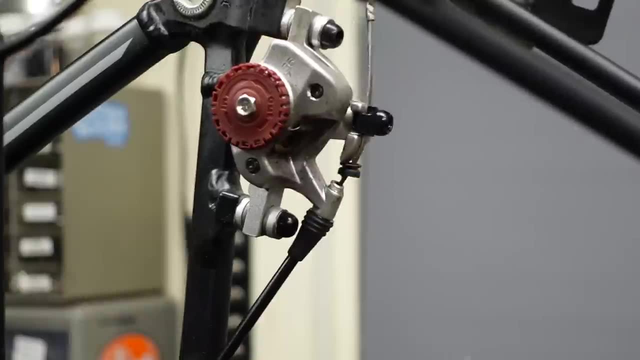 You just drop some lube And then work the lever. Now, if this felt really gooey or sticky or grungy, I'd definitely pull it, clean it, replace it, do what it takes, But it feels really good. So this is just kind of preventative. 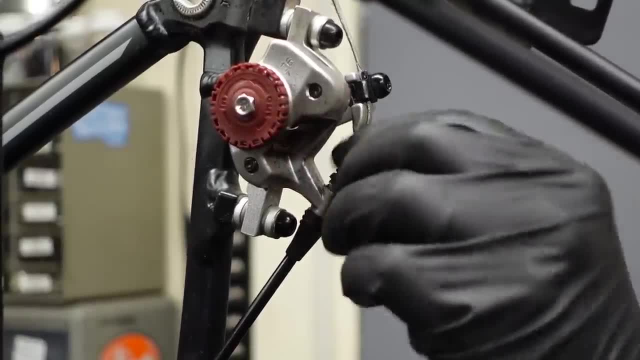 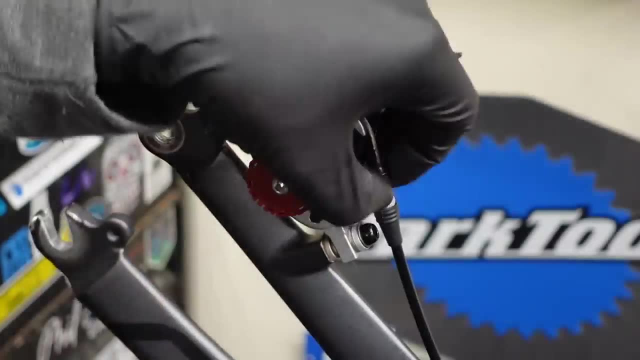 And that's one spot, And we can do the same to the front. Don't forget to put your seal back. the way you found it Keeps the dust and grime out of there. So yeah, obviously this is a lot easier when you have a bike repair stand. 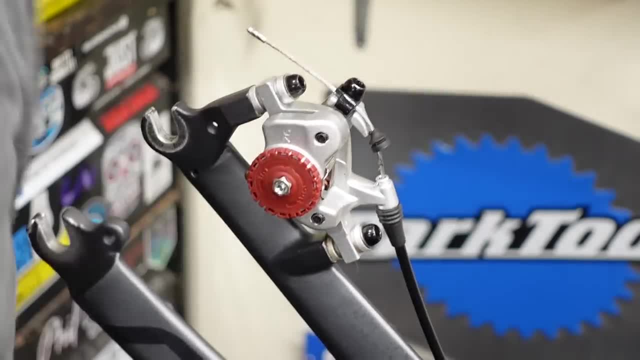 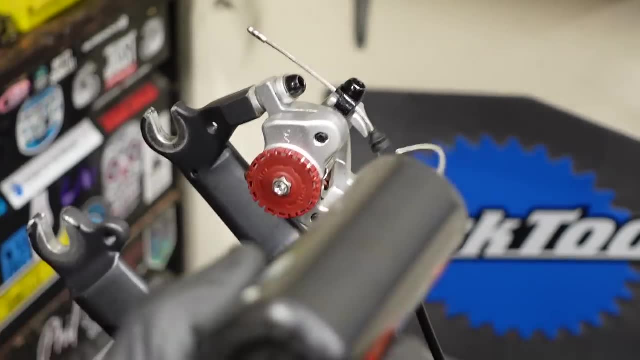 You know, if you're an avid cyclist, you should probably have one. Get yourself a good folding stand from Park Tool. Keep it in your garage. This isn't something you need to do before every ride, But I definitely go through my bikes regularly. 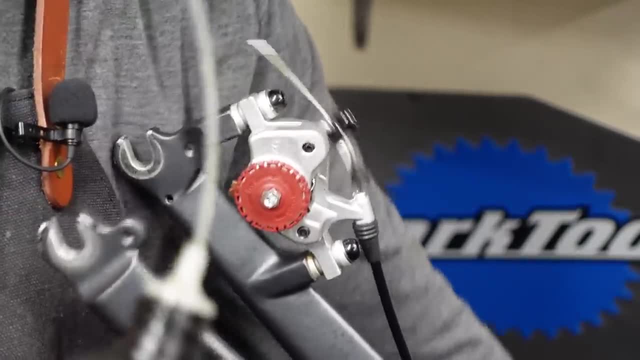 You know, before every big ride, Just to make sure that everything's in the right place, I just go through it and I'll drop, you know, a couple drops of lube here and there, And then my bike's always working perfectly. 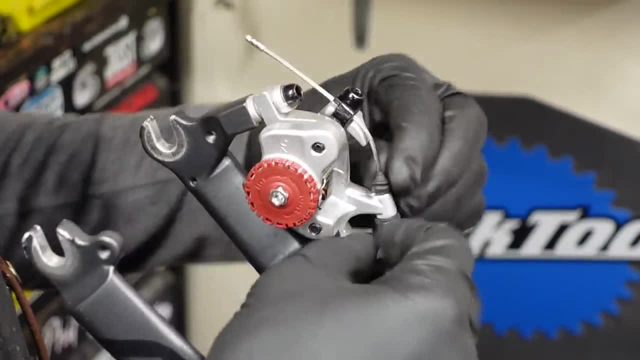 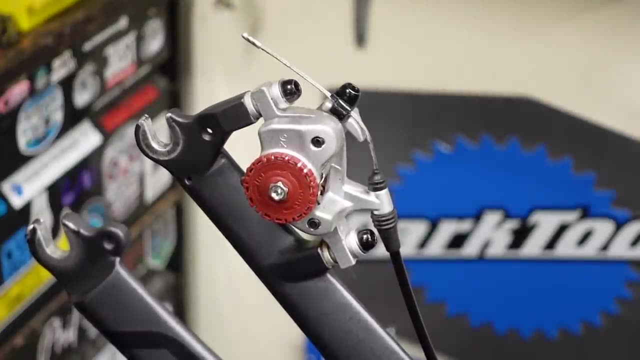 And you know. really it's only. It only takes like once you get used to doing it and know what you're doing, it takes 15 minutes to go through a bike And keep it clean And lubed up. 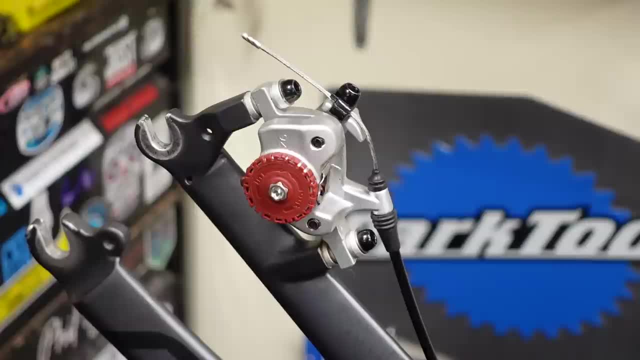 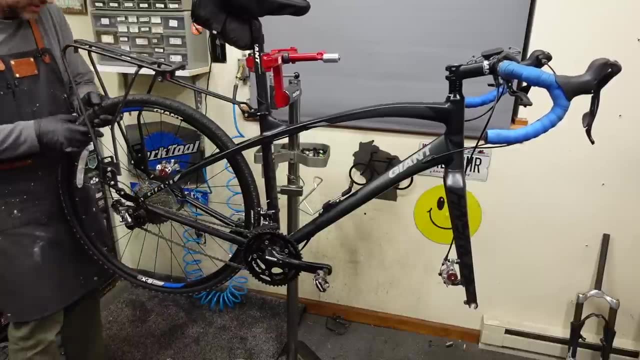 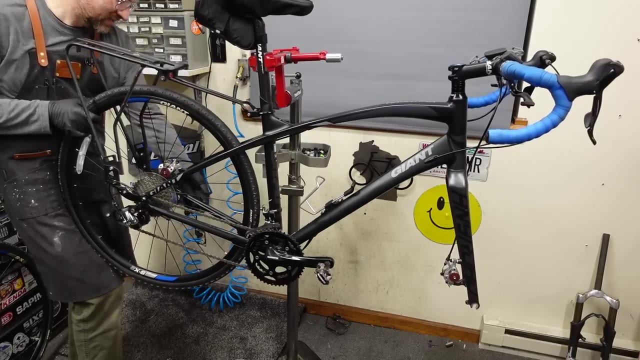 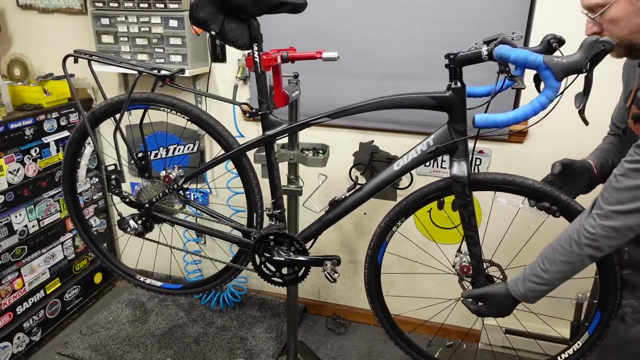 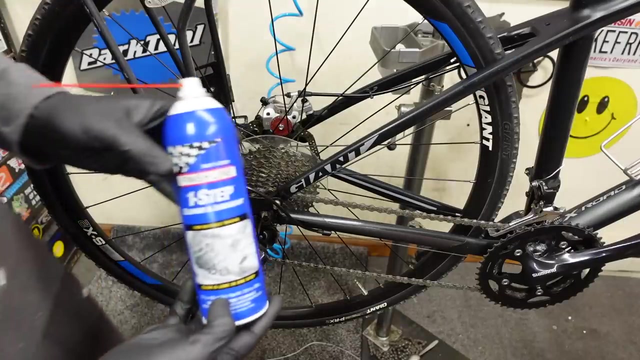 You know, it's preventative maintenance. Really simple, But something you can easily do at home. Clean bike And clean wheels: We'll put them together and we'll have ourselves a bicycle. I'm going to use a little bit of One Step on this chain. 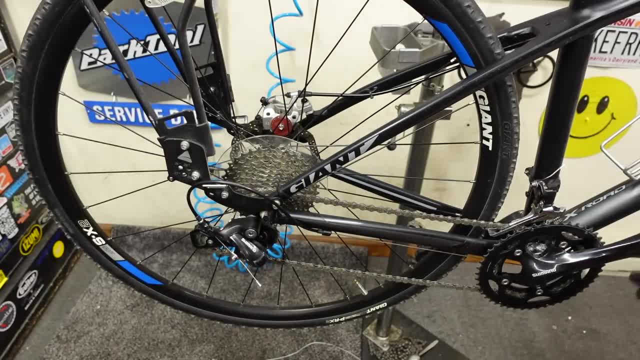 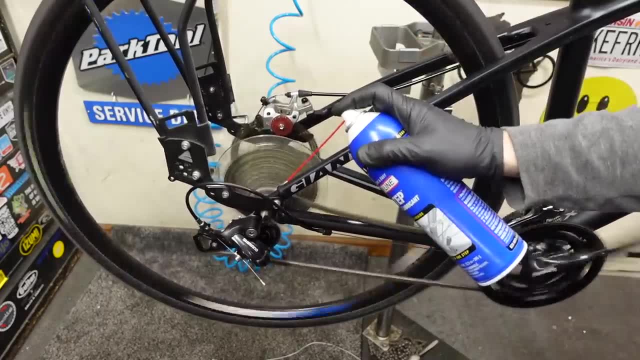 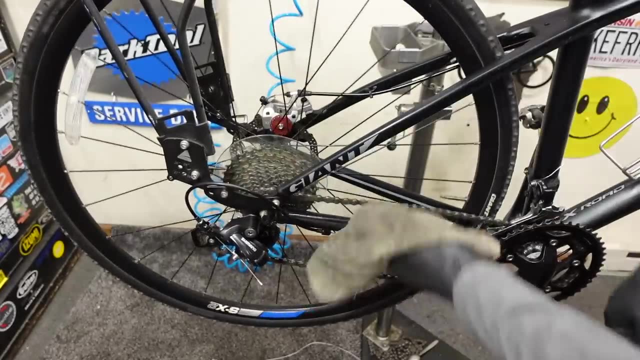 It's a cleaner and lubricant. Just because the chain is mostly dusty And it's a little dry, I just spray some on there And I'm going in the. I'm in the high gear Because any of the spray from the aerosol keeps it off that disc. 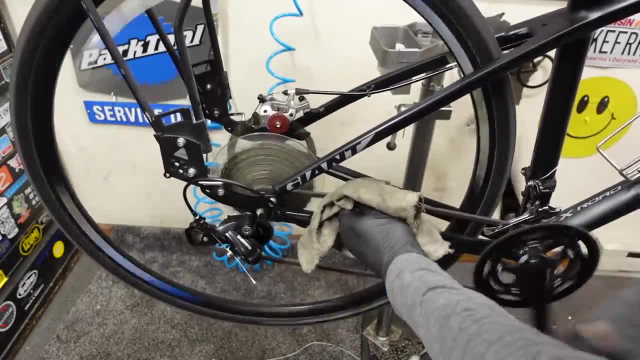 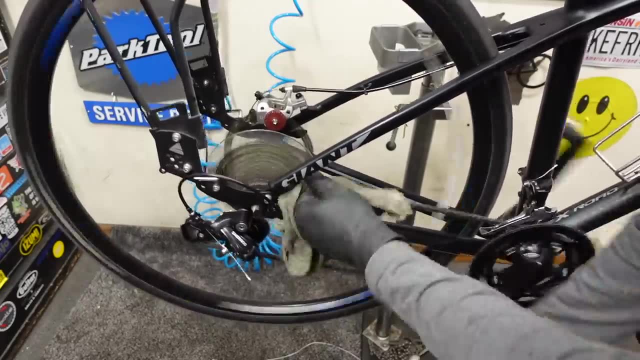 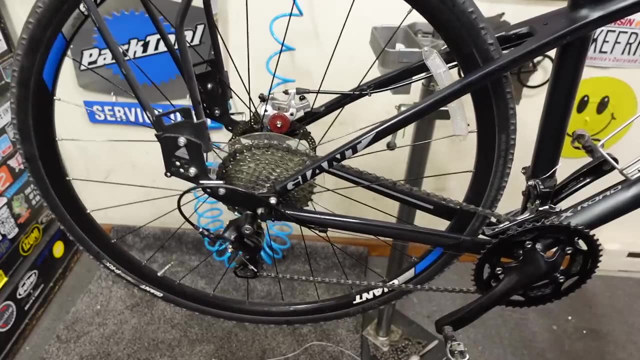 I know that's going to get some. That's going to get some comments. It's a trigger point for a lot of you. And then I shift all the way up into the low gear And then, without pedaling, I click the lever to loosen the cable. 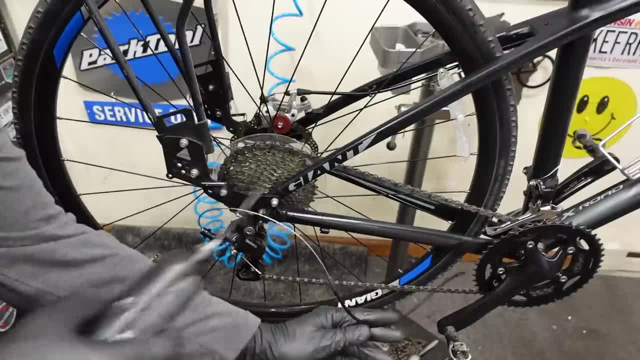 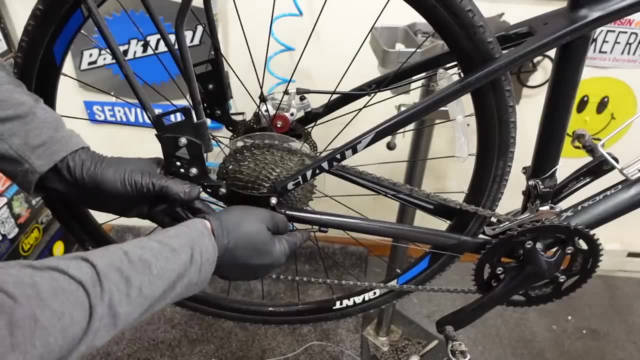 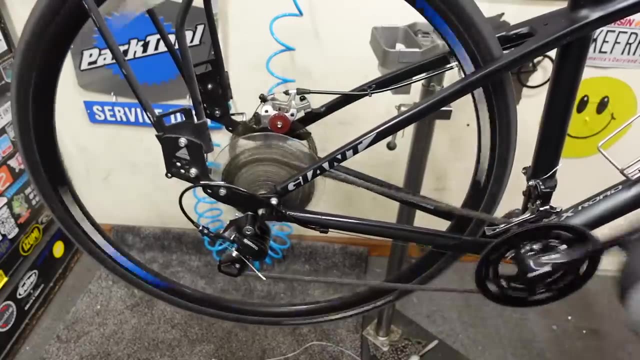 And I can pull this piece of housing out. Once you get this piece of housing out, you can lubricate that a little bit And that makes things slicker than snot on a doorknob. There's definitely something going on with the shifting here. 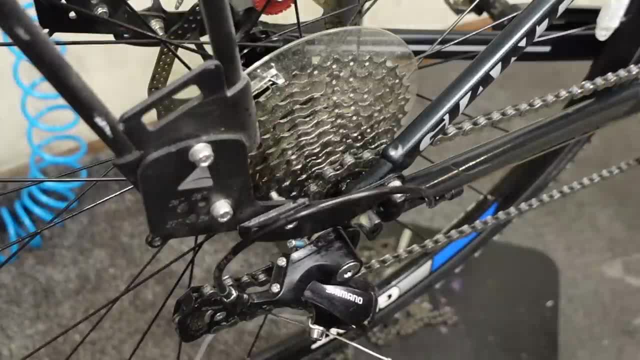 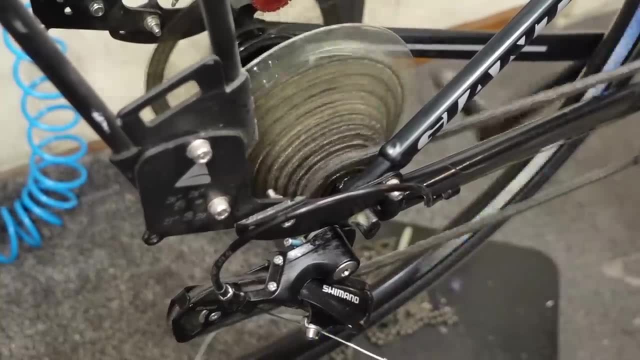 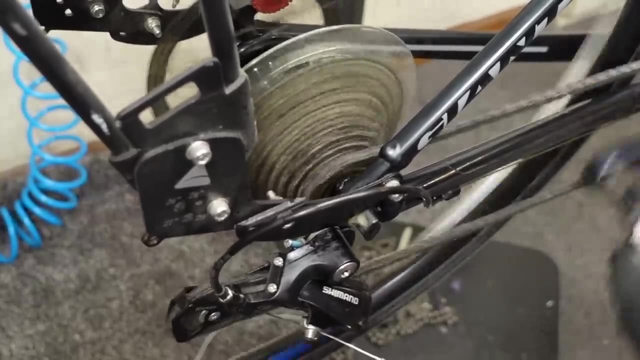 Let's take a closer look. I'll try to walk you through what I'm doing here, What I'm looking at. So I'm in the high gear, Okay, so I just shifted once up, Okay, and it's struggling to go up. 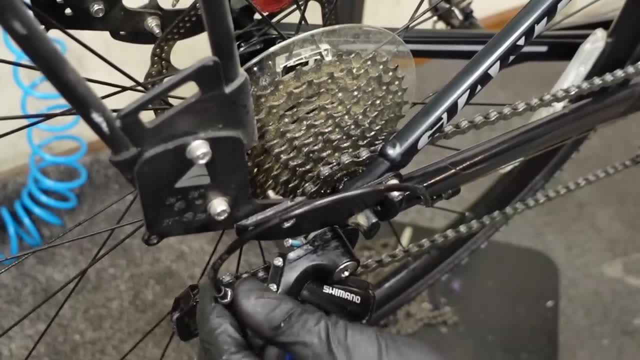 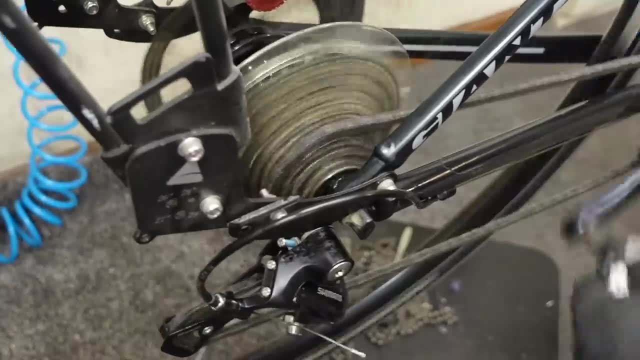 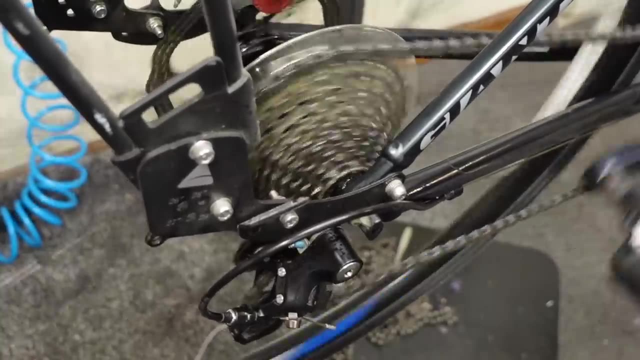 And I can feel my cable tension is a little low. So back the barrel adjuster out a smidge. Three, four, Okay, now it's shifting nice and crisp, Very smooth. Okay, I'm all the way up into the low gear. 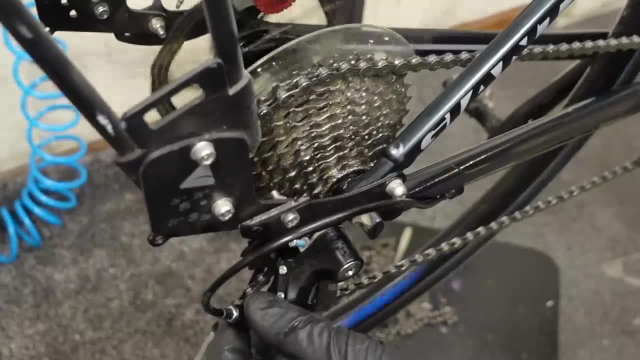 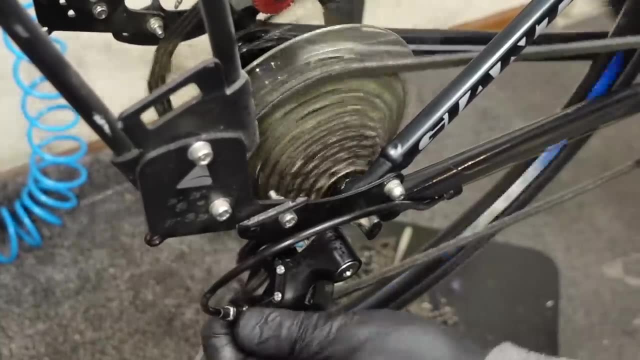 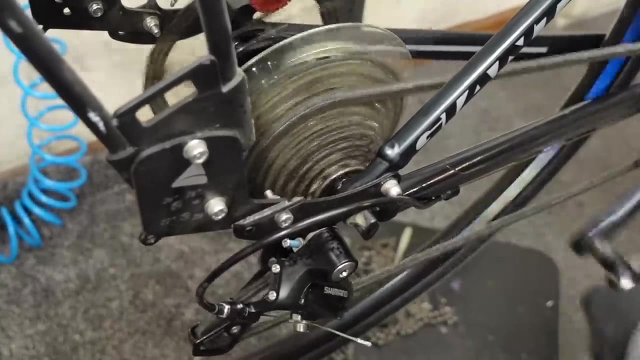 Back down. I'm hearing a little bit- And it's not just the front derailleur Feeling Okay. so I'm just turning the barrel adjuster in like a quarter turn, Just dialing it in Because there's Hey, the bike is shifting and accessing all the gears. 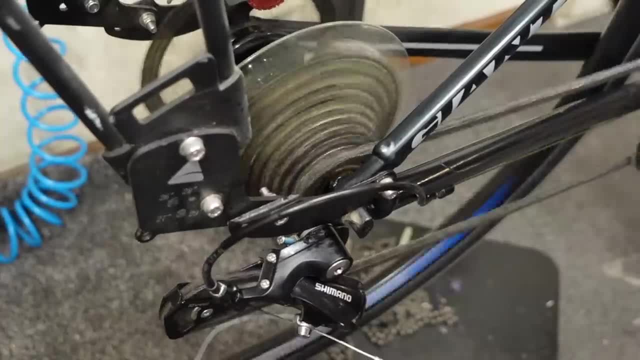 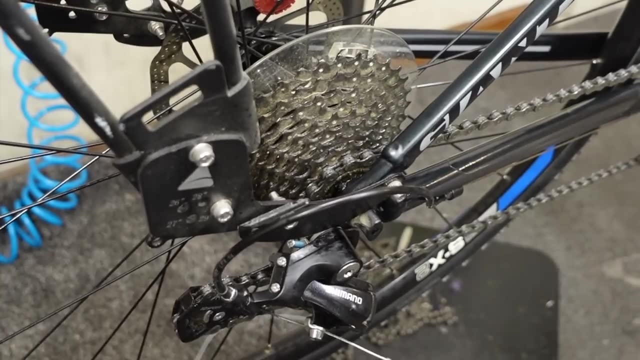 And then there's tuned, And I'm here for a tune-up, So I'm going to make it just right. That doesn't feel perfect. I don't know how to explain it to you. You should get a JIS-2 screwdriver. 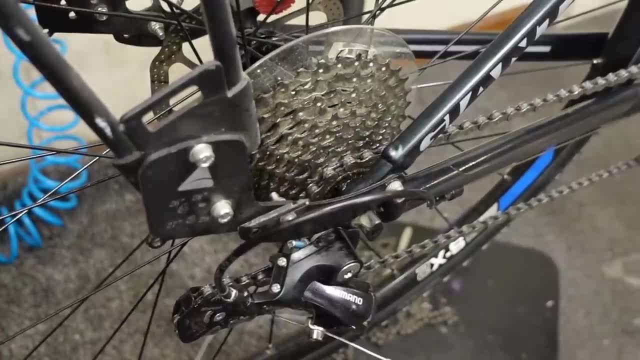 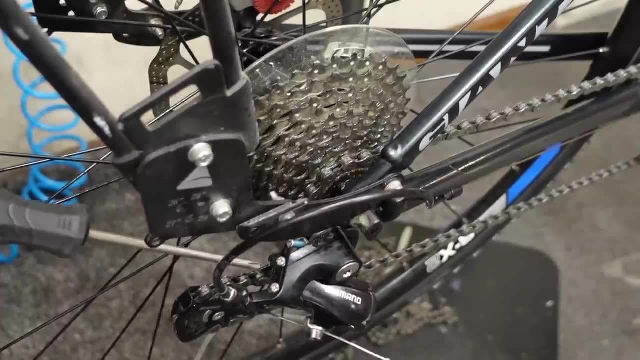 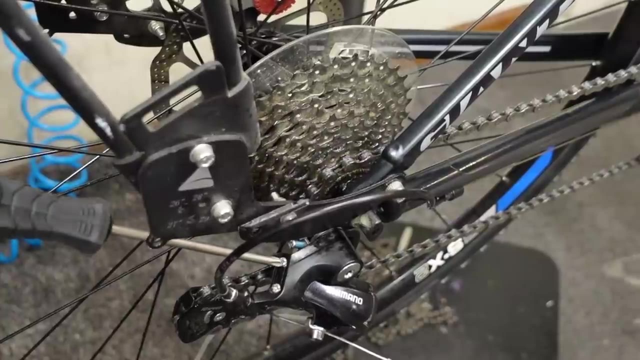 A regular Phillips will work, But the JIS-2s are better. And then these screws- here are your limit screws. There's a high and a low, They have a little H and an L, And this is the high gear. Even though it's on the low part of the cassette, it's the high gear. 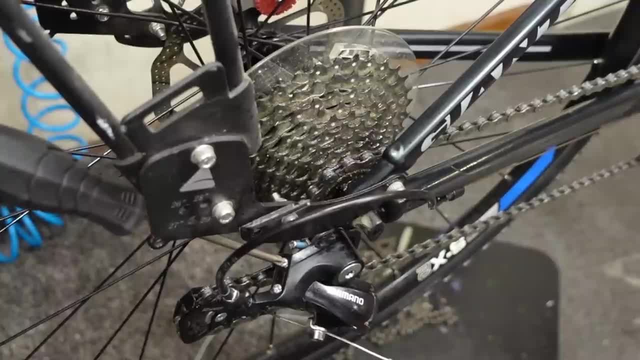 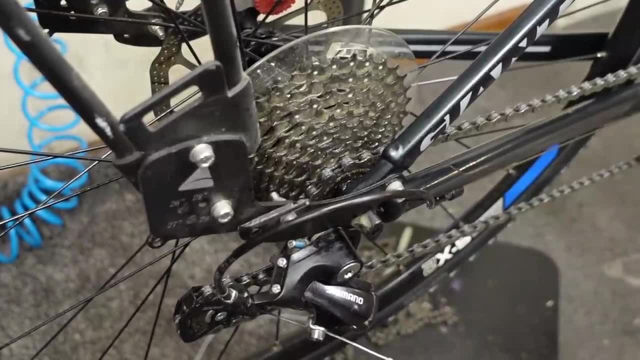 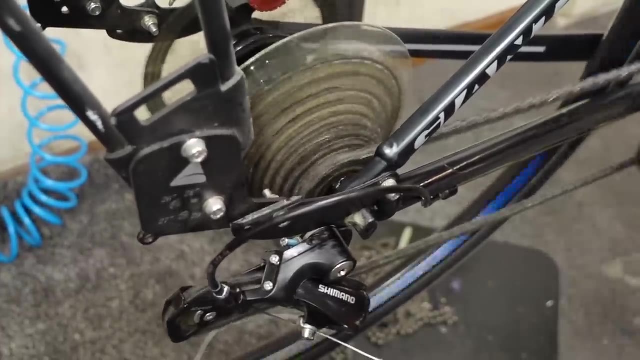 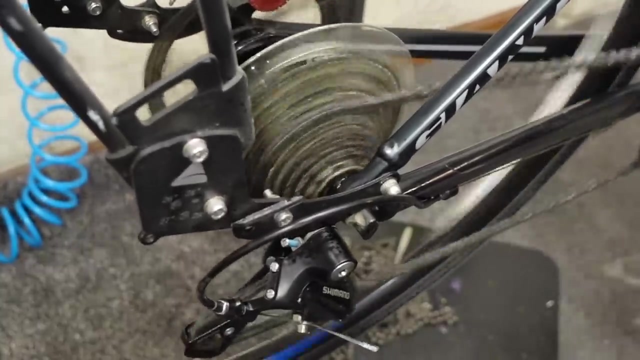 It's the little one And I'm just going to back it off that much. That was like a half a turn, And I'm doing that because it was making noise, And it's probably only a noise that someone with my level of experience can hear. 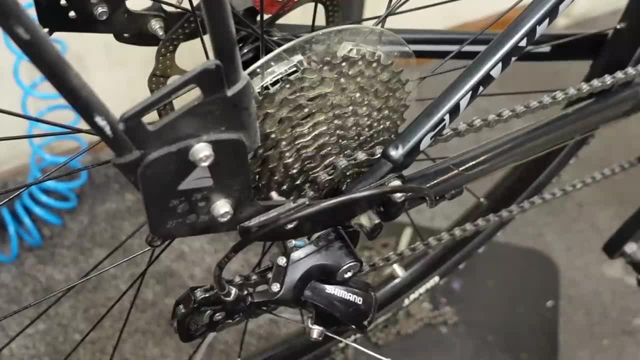 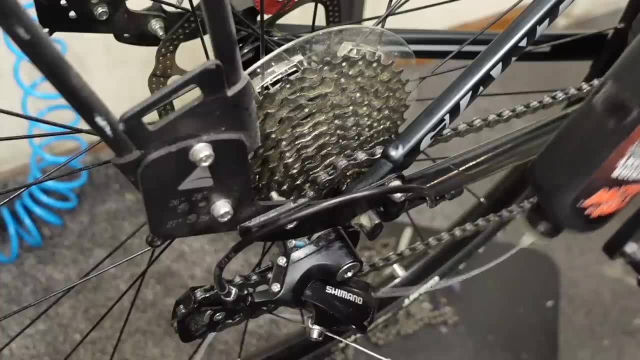 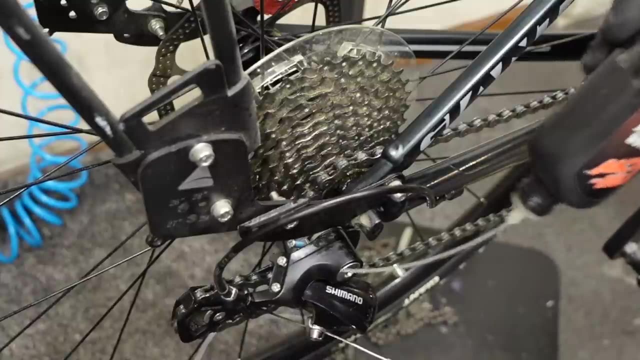 But that was a very, very minor improvement I made, Just because I'm going to drop a little bit of lube. There isn't any lube coming out of this bottle. Oh, there we go. Something was gumming up the works. 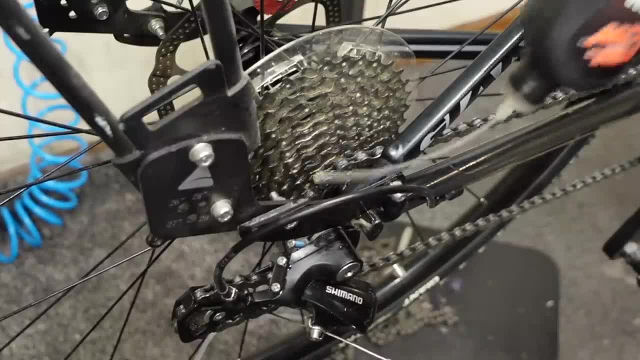 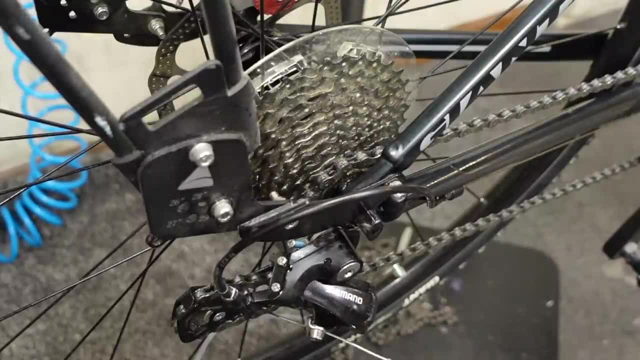 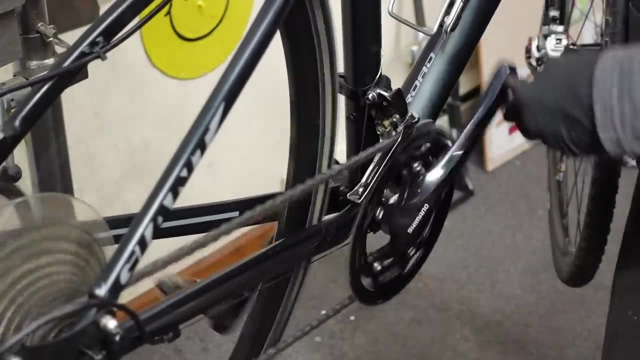 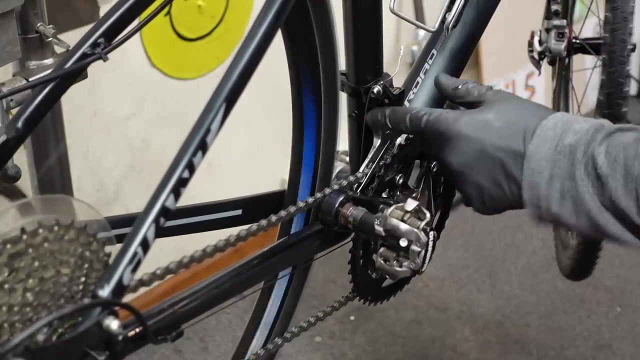 And I'm just kind of dropping lube all over things here. This just helps keep the rust at bay. So now I'm hoping to focus in on the front derailleur here. All right, It's a two-by And there's a little bit of slack in the cable. 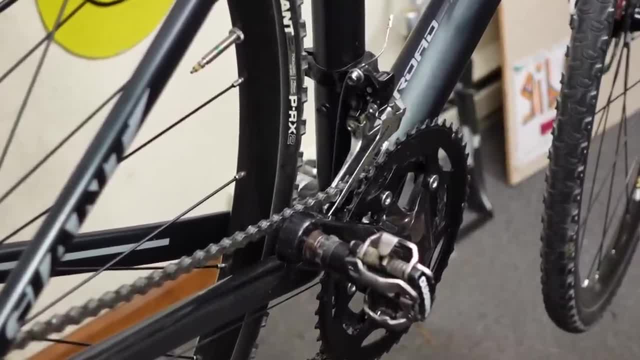 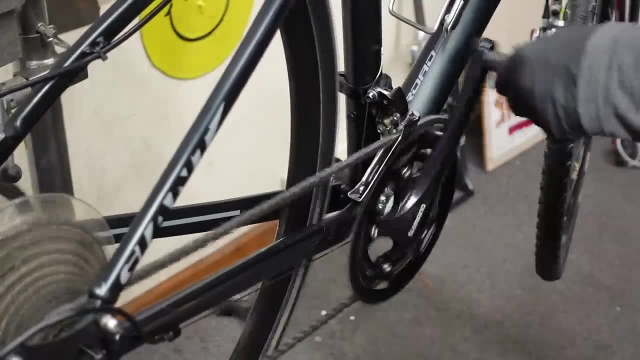 There's a barrel adjuster up at the lever. I'm going to turn that out a full turn And that will pull that cable a little bit tighter, And that's all it needed. So I'm in the high gear back here and the high gear up front. 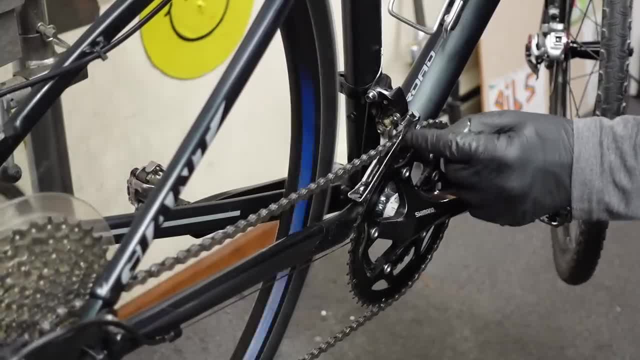 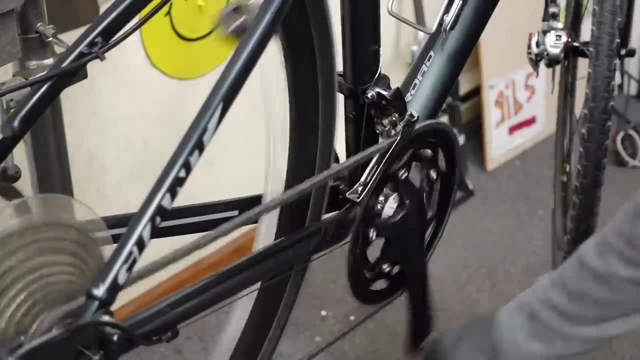 So this is the very highest gear which the chain is going to want to rub on the outside of the derailleur, the inside part of the outside derailleur cable or derailleur cage, And it's not anymore. Then there's a trim shift halfway. 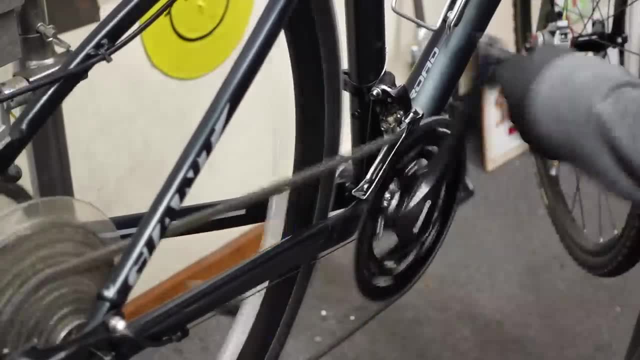 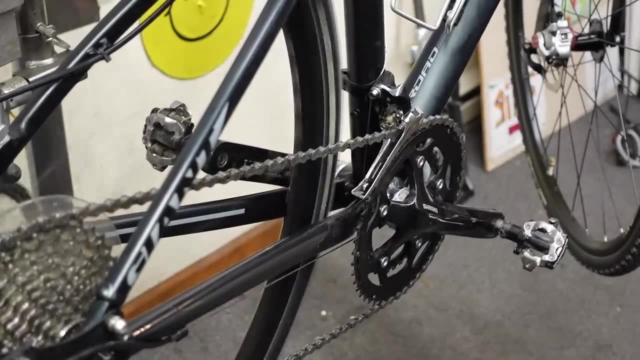 which will move it just a smidge, And that's fine. Okay, And now it's not rubbing when you're cross-chained. Now everybody will tell you not to cross-chain And it's preferable to not cross-chain, But you can do it. 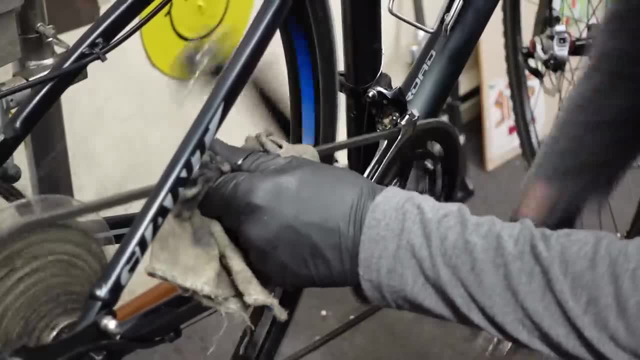 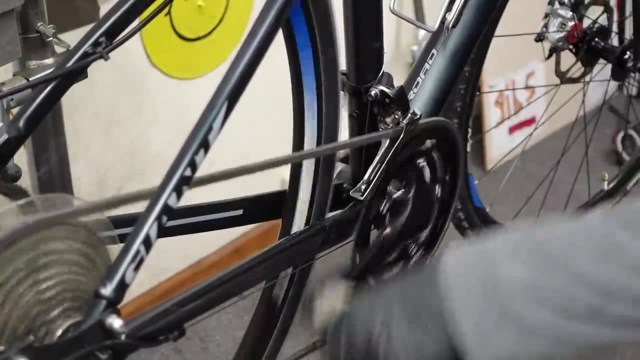 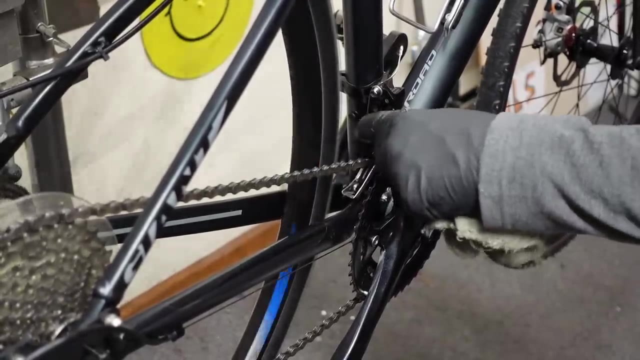 It's not going to break anything. It's just going to wear things out faster And it's not the happiest state the drivetrain will ever be in, But it's not a sin. Okay, Now we're in the granny gear, And now it's going to want to rub on the inside part of the inside derailleur cage. 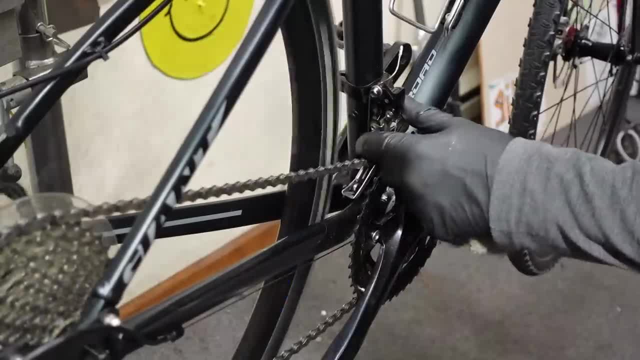 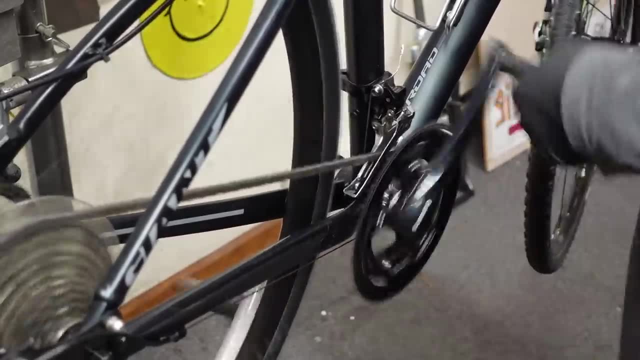 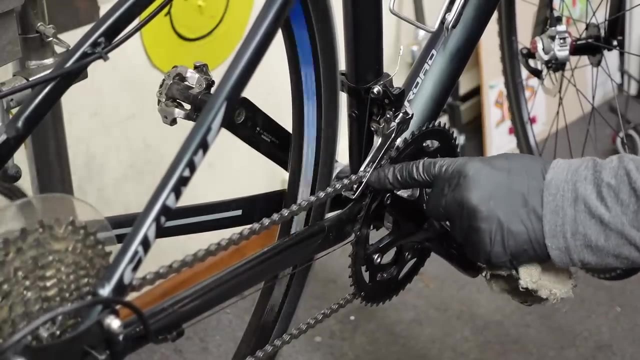 And that looks really good. So no adjustment needed there. Then we're going to check little and little Cross-chain the other way And you're going to expect a little bit of rubbing there. So it's rubbing the inside of the outer cage. 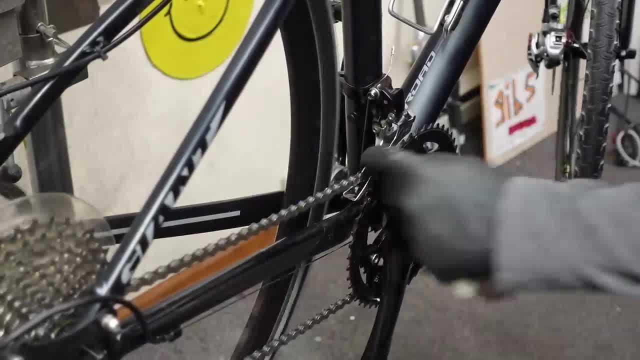 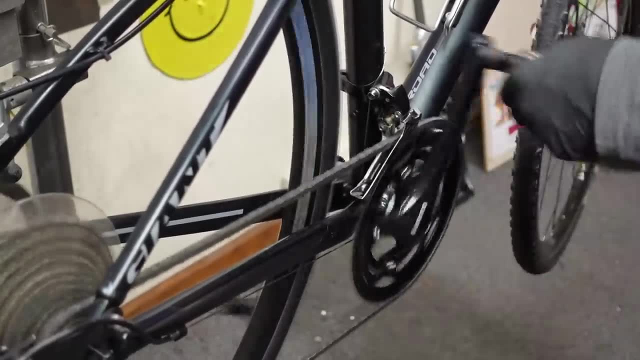 But there's a trim shift, So if you push your lever over halfway, it moves the derailleur halfway, And now you're cross-chained and not rubbing, So this is perfectly adjusted. I absolutely love this drivetrain and how it's functioning. 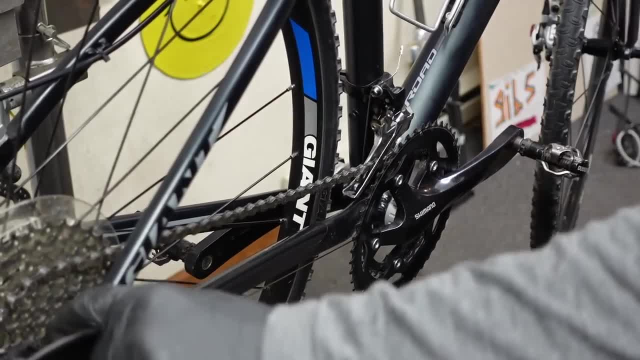 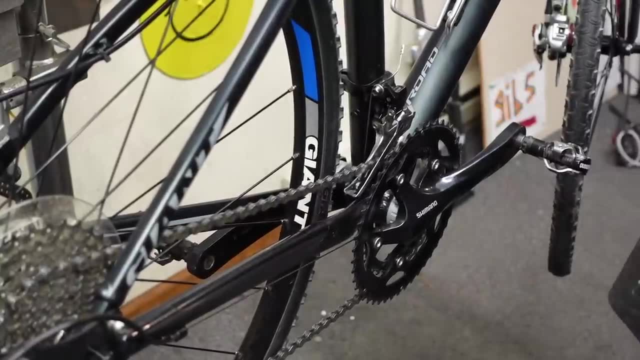 And it's not. I don't even know how many speeds it is: 1,, 2,, 3,, 4,, 5,, 6,, 7,, 8,, 9,, 10 speed Shimano. It's working great. 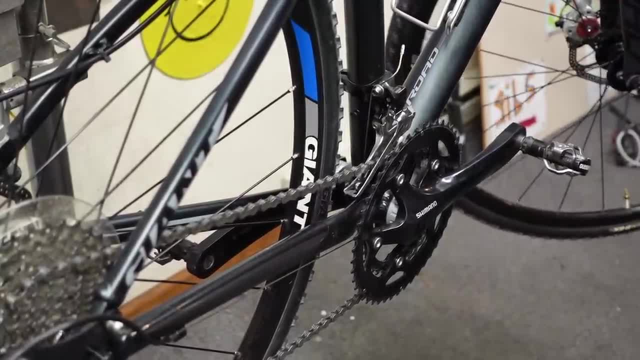 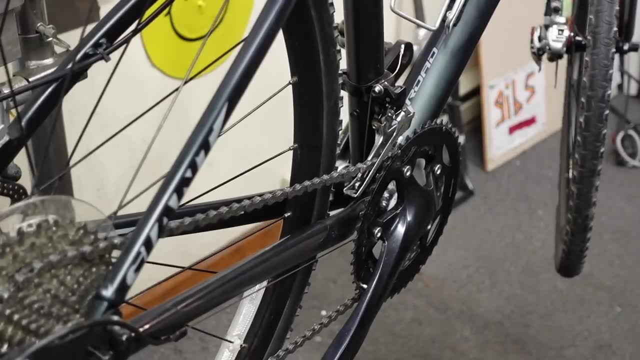 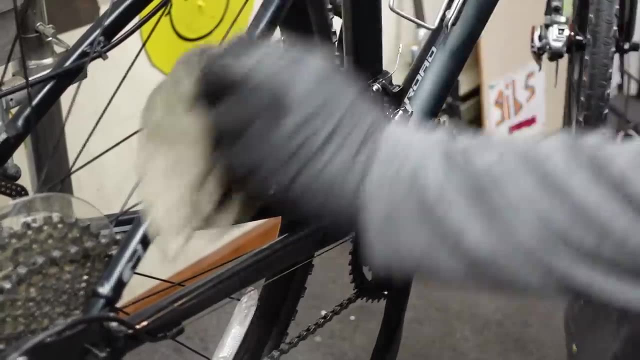 Imagine that, Yeah, It says Shimano 10 speed on it. It's not Claris, It's not anything, It's just generic Shimano stuff And it's great, It's wonderful, I love it. You know, Some people would say it's cheap garbage. 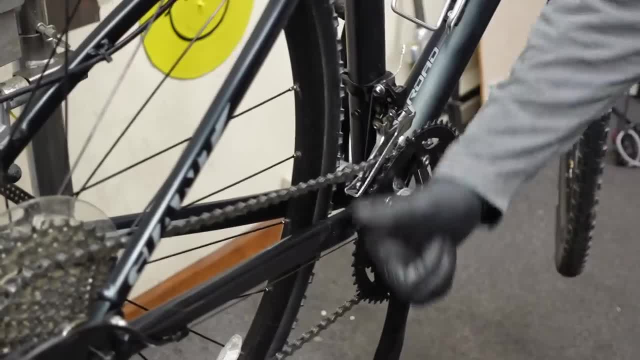 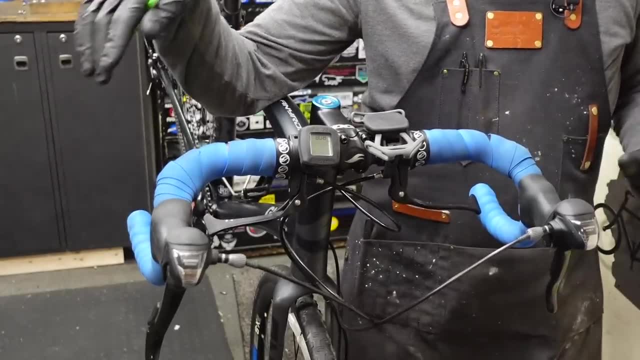 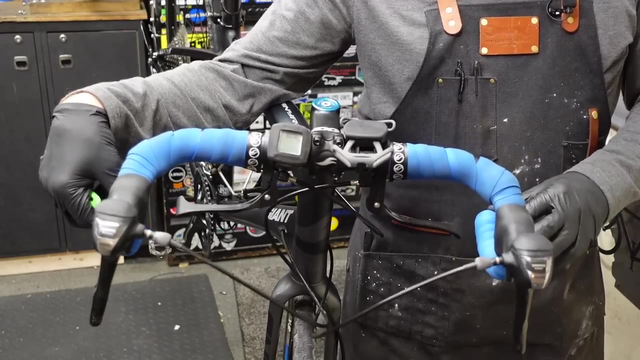 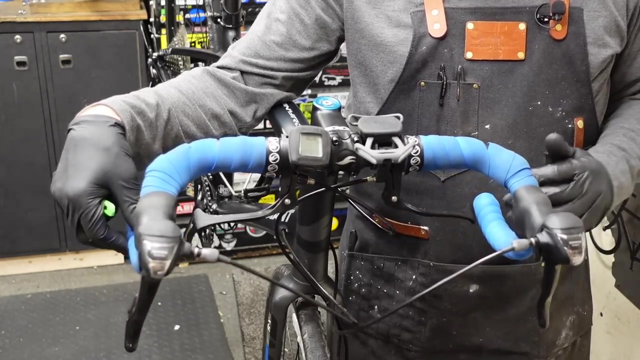 But it's definitely not. This is good, good stuff. Love that. So this is something that I see all the time on bikes that are owned and ridden but not maintained By the owner, which is not something that I expect, But you know, I mean these are easy things that I feel like anybody should be able to. 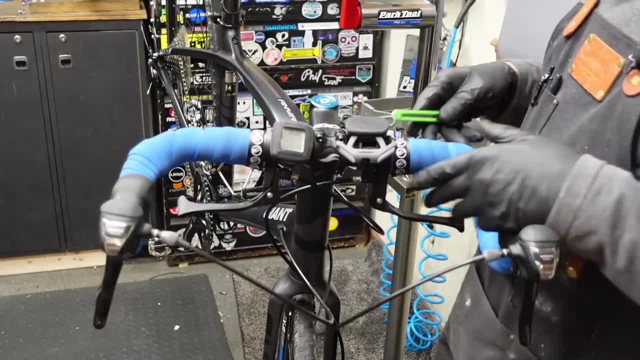 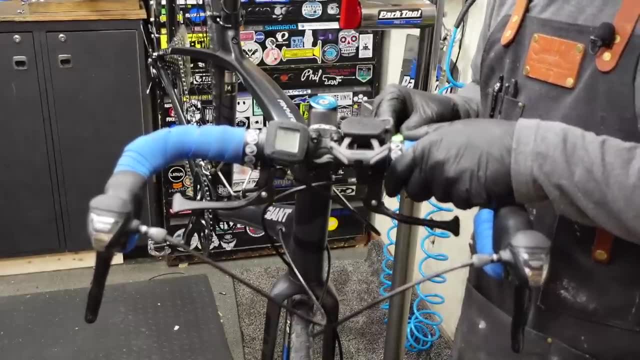 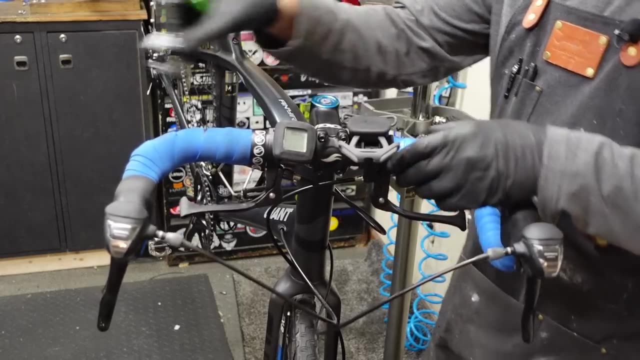 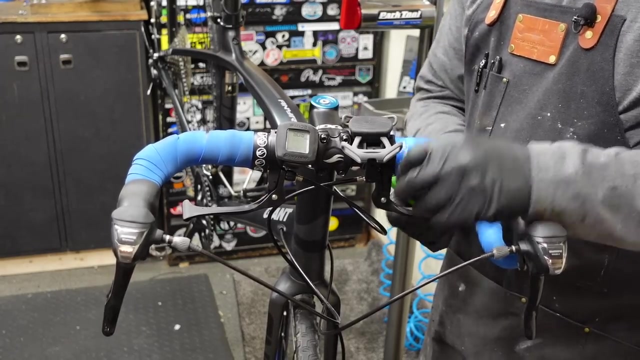 do on their own with relatively little effort. But keeping your tape from sliding around on the bars is pretty simple. I'm just taking a little utility knife here and cutting the finishing tape and removing just the finishing tape. Okay, You want to be careful that you're not like cutting through the main tape. 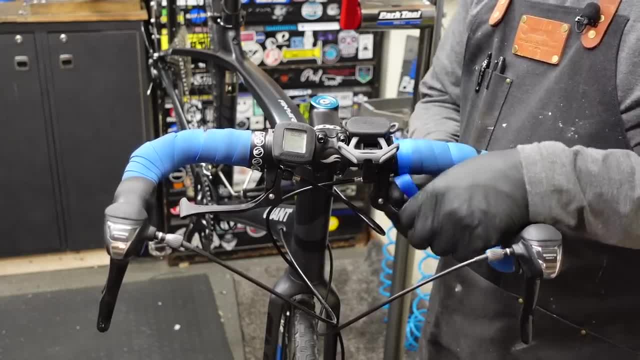 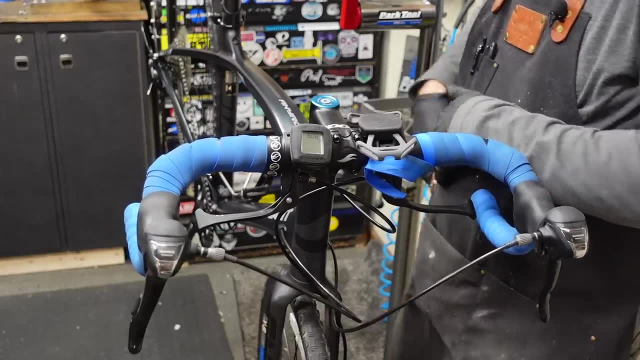 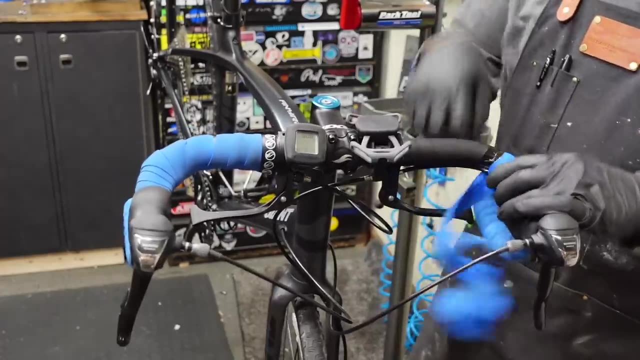 So this is more finishing tape. Okay, So now we're down to the bar tape, And you can see this is already cut into a wedge, And all I'm going to do is unwrap it until we get to the hood, where it looks like you. 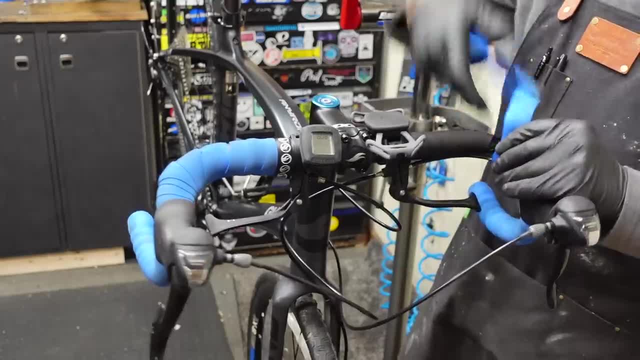 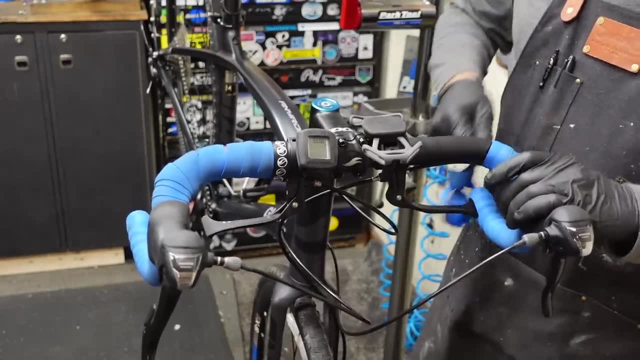 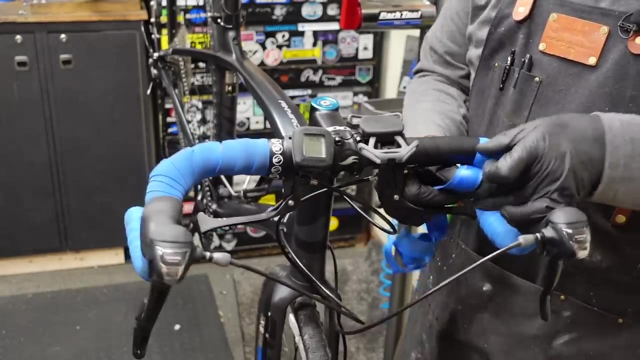 know, this stuff is all kind of stayed put. You know, part of the problem is is with this cheap cork tape there's no sticky on the back, So it is going to slide around, It's going to want to, And I'm just pulling with a moderate amount of pressure here. 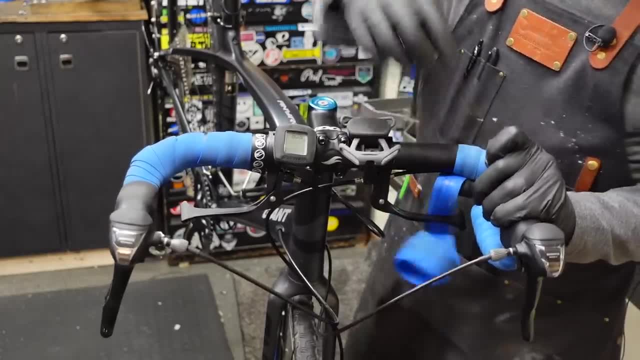 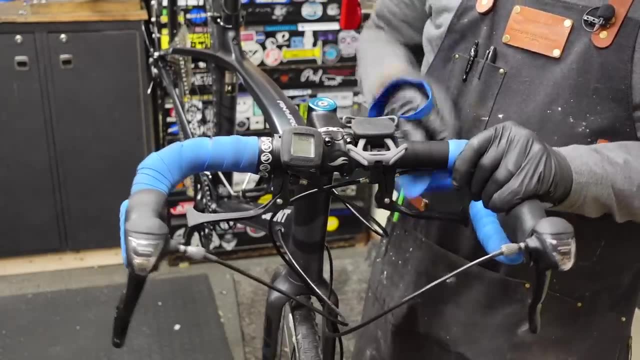 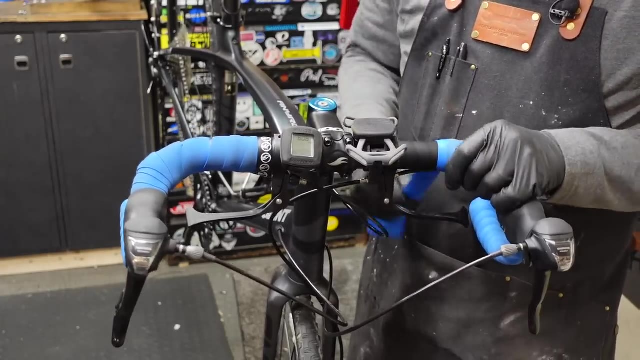 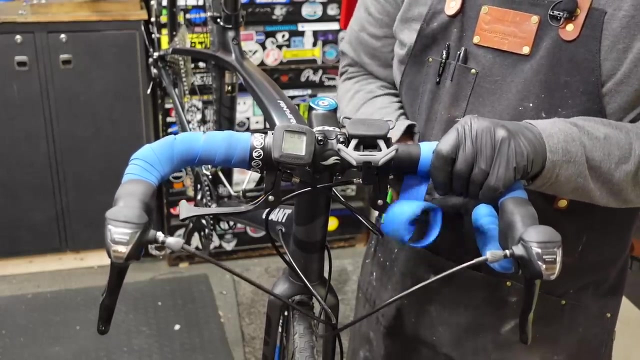 And then I would say about halfway on each layer. I'm going halfway, Try to keep things evenly spaced so it looks good. And I'm just going around and around Constant, consistent pressure Or tension. I should say One wrap at a time. 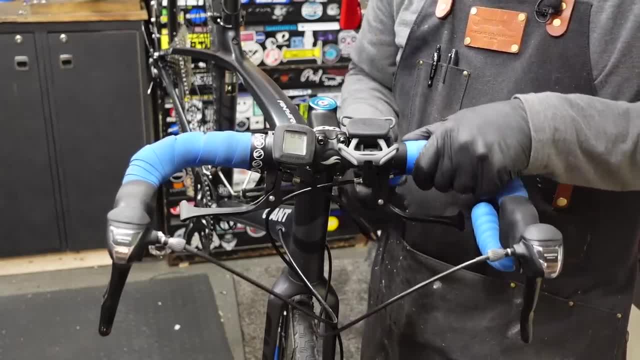 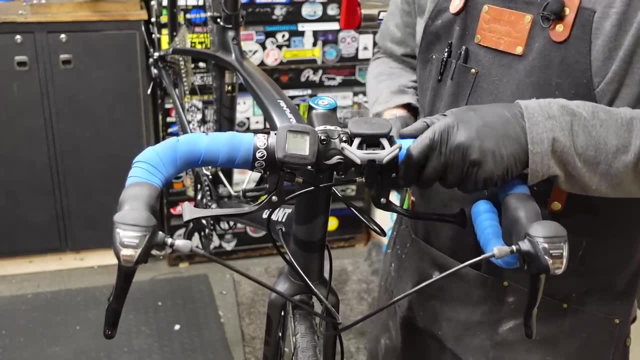 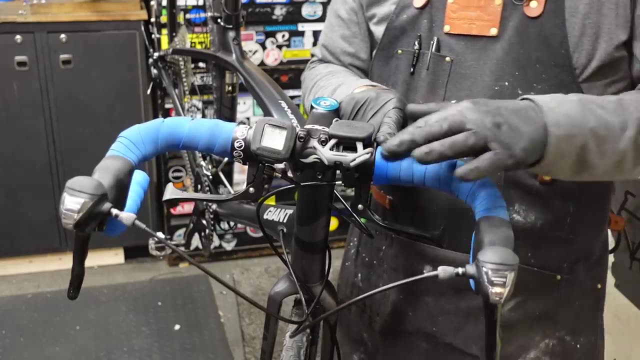 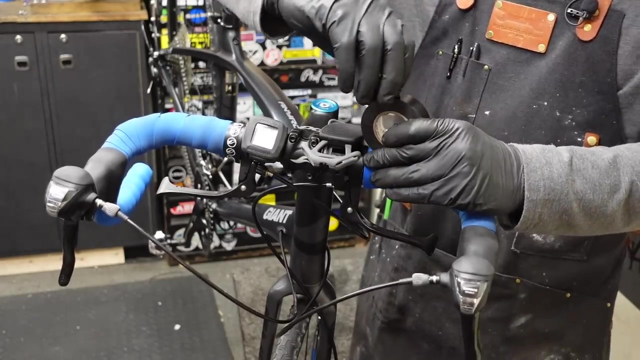 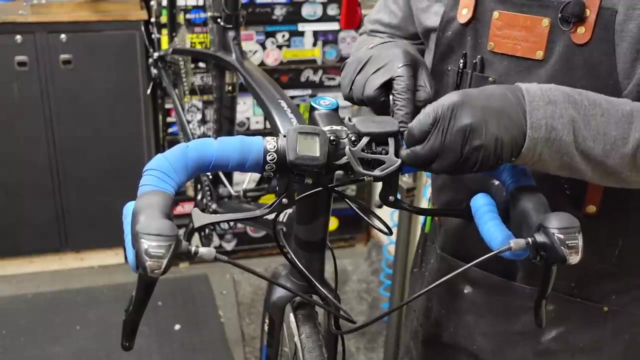 Nobody's in a hurry. Get to the end here, Okay. And he's got an accessory And you can see it's nice and even Okay. Then I have nice electrical tape. I don't use the cheap stuff. Cheap stuff just gets gooey and fails. 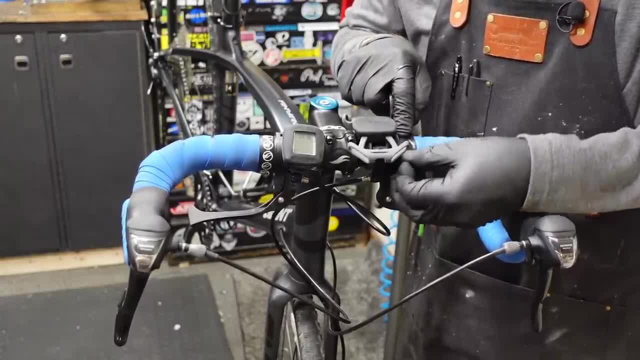 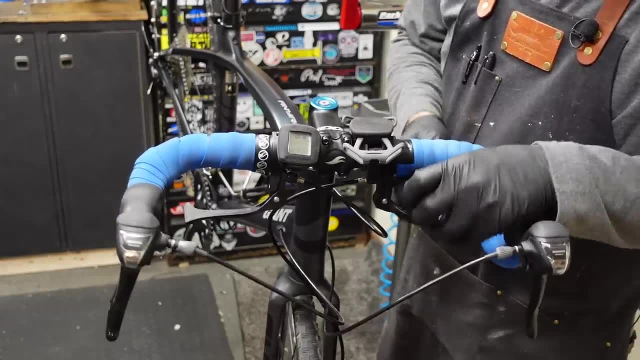 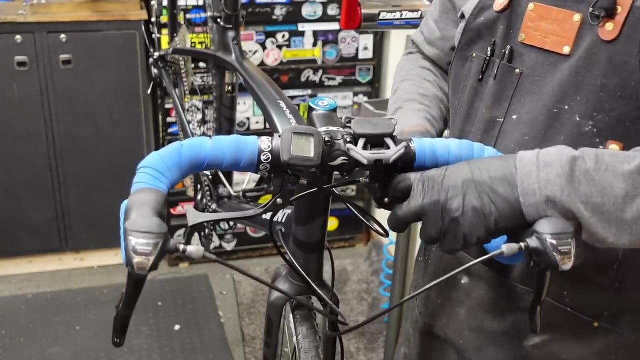 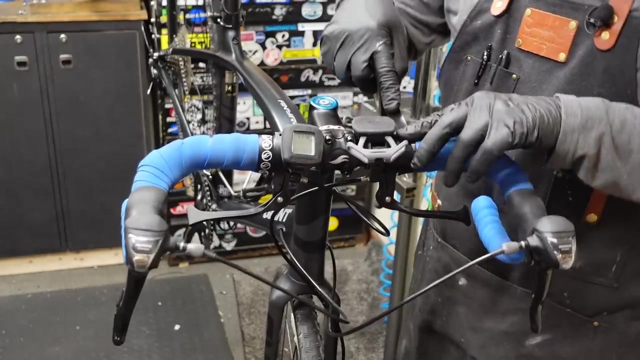 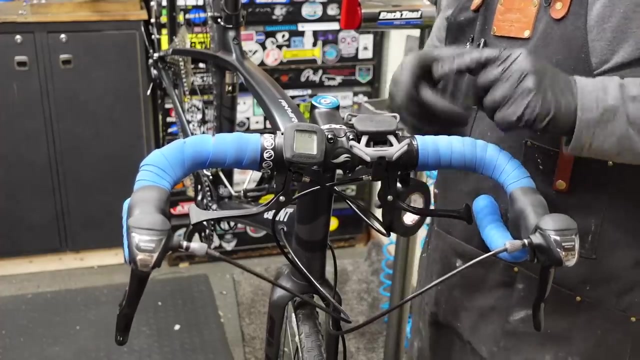 Pay extra and get the good stuff Only a couple bucks And the first two laps around I'm pulling pretty tight And then I like to only have one layer. I don't like to wrap electrical tape like the other stuff, It's just one thickness of it. 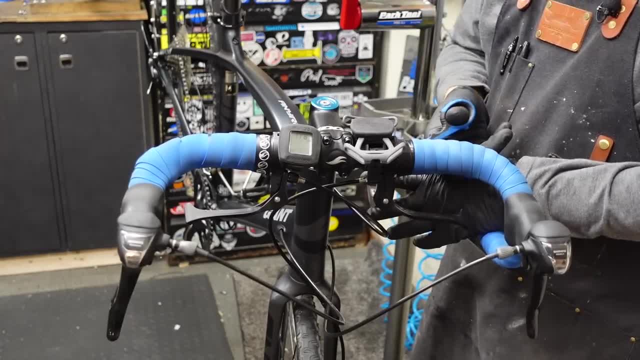 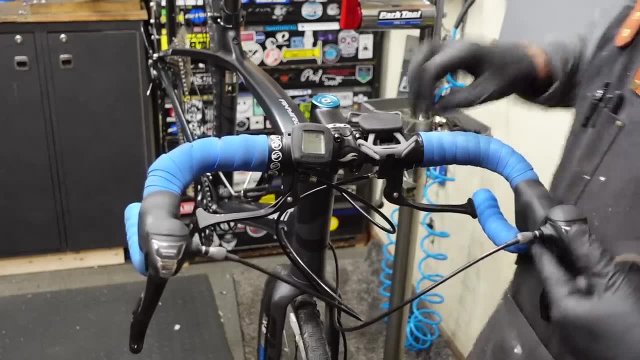 But if you don't pull it super tight, then it's a little bit wider and it covers up all the stuff that you pulled super tight. And I always like to finish it where it finishes- underneath, And then you know, because your fingers don't really get underneath. 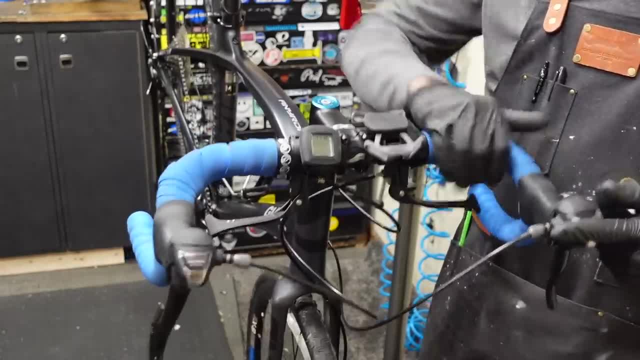 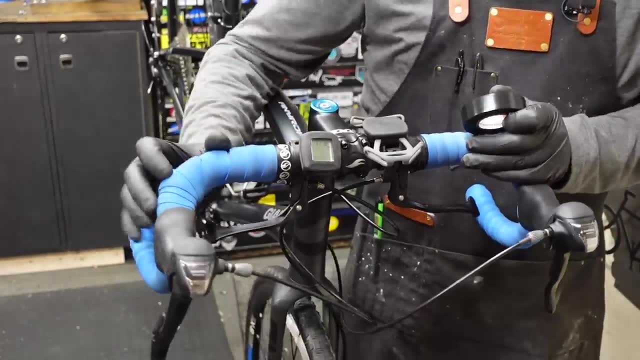 And so it usually stays put then And now that you know, because people like to ride up here And they're putting all kinds of pressure outward all the time And that's why it slides. But I think I've got that wrapped a little tighter now. 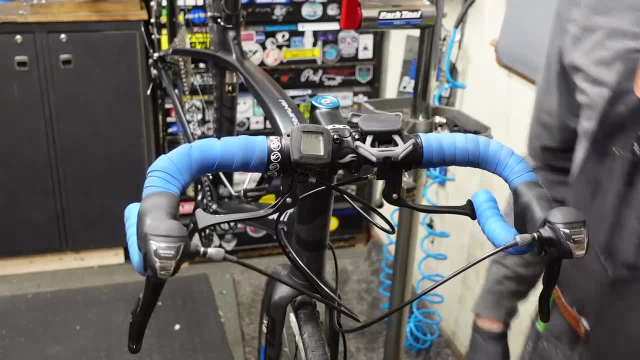 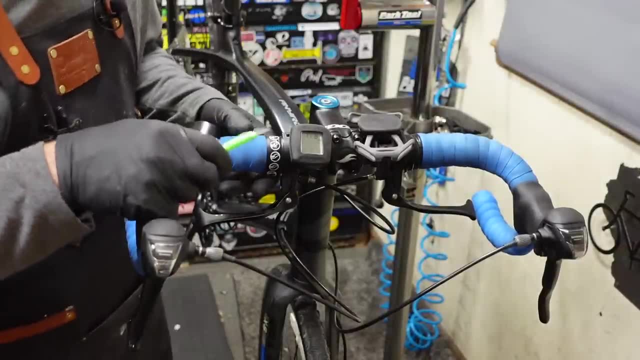 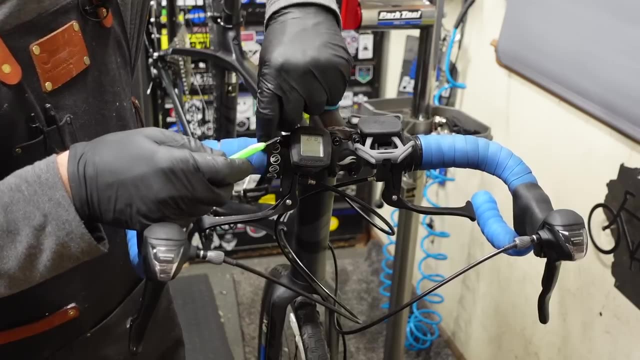 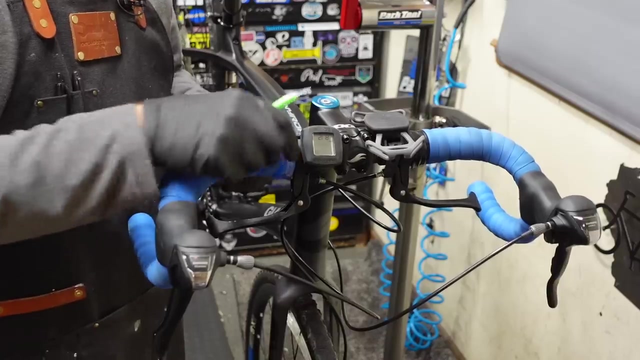 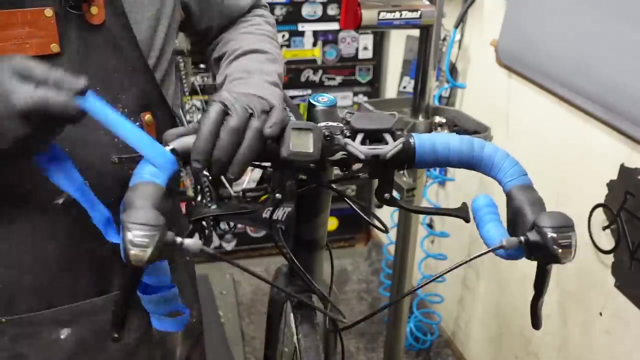 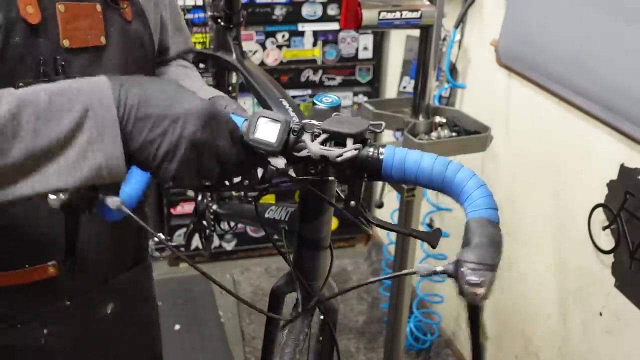 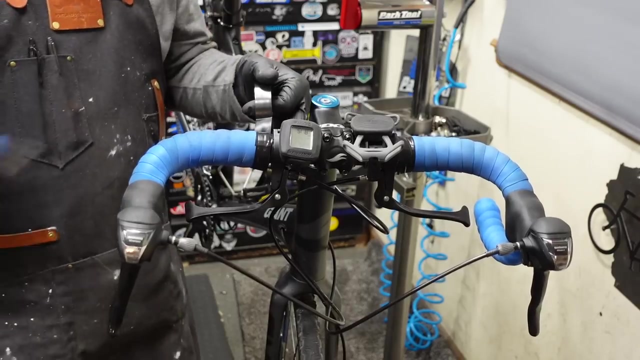 So hopefully it prevents that from happening in the future. Yeah, this is the only tricky part really is the finishing tape. You just want to make sure that you're not cutting your bar tape. Yeah, it's kind of hard to get the first time. 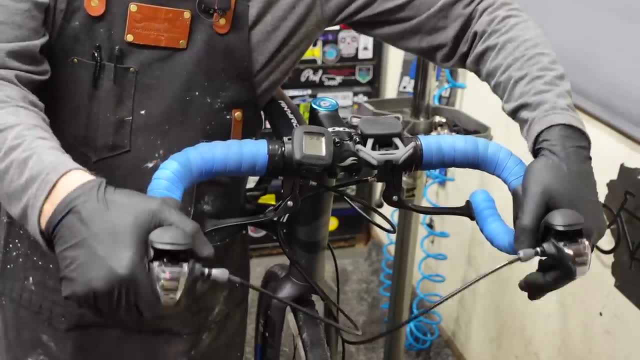 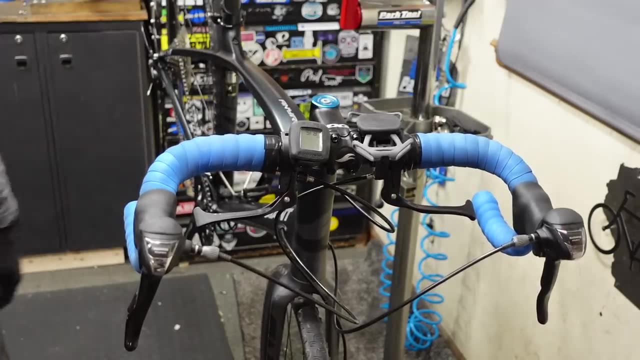 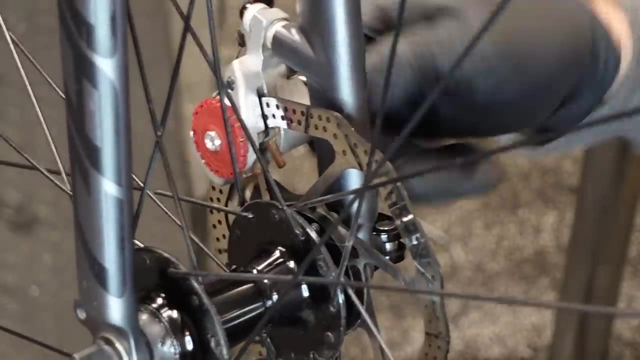 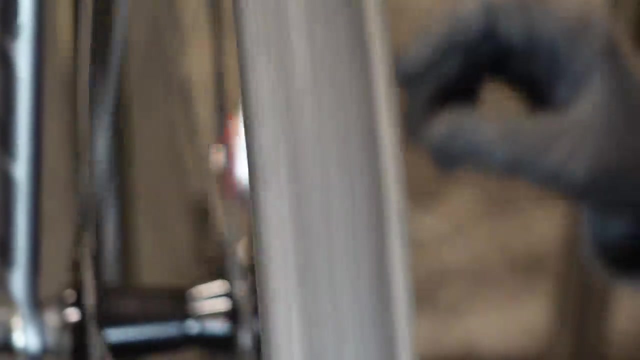 Yeah, the brakes feel really good. No adjustment really needed there. Oh, but that front one's rubbing. Let's take a look at that. well, this has a pad adjustment too. I can use the pad adjustment, okay, so we're gonna turn that pad. 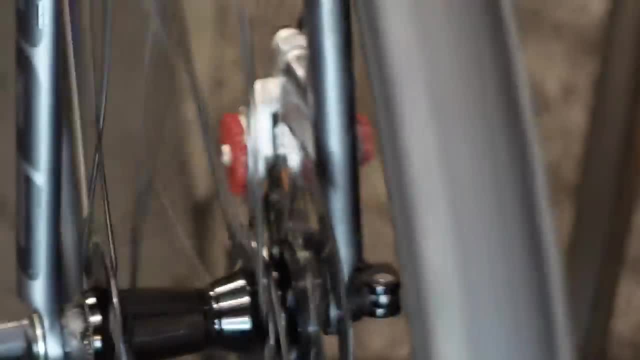 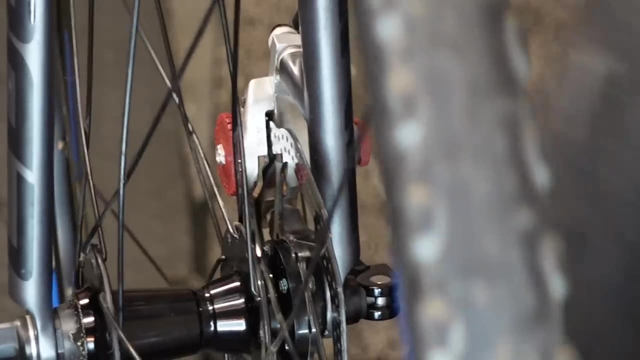 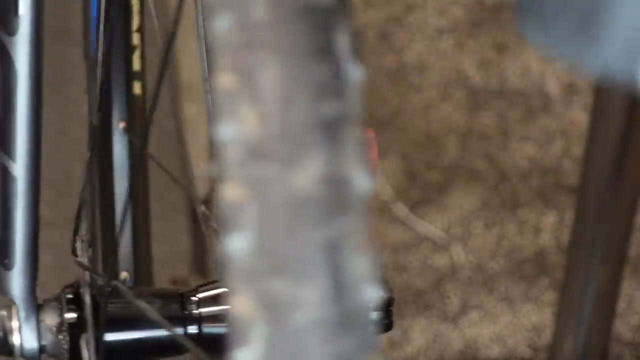 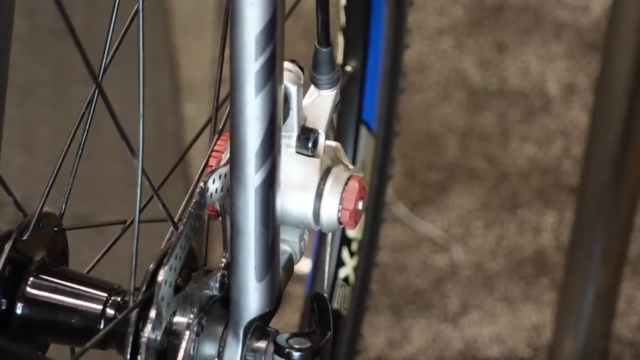 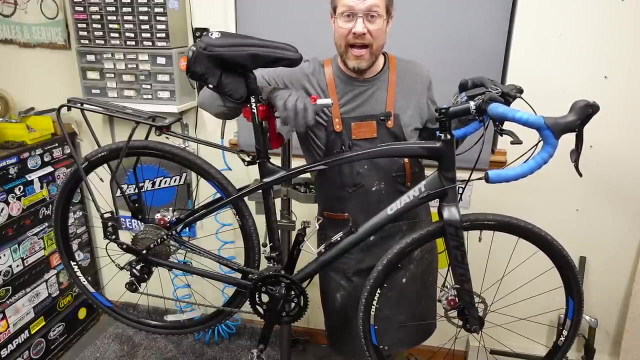 in a little bit. oh, there you go: pad adjustment. so you have a pad adjustment here and here. that's as good as I'm gonna get it. well, there you have it. bike farmers, it's a pretty straightforward tune-up. if you're an avid rider and you're riding a lot, there's little things. 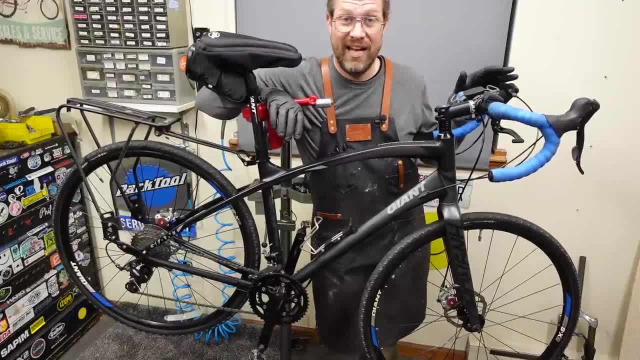 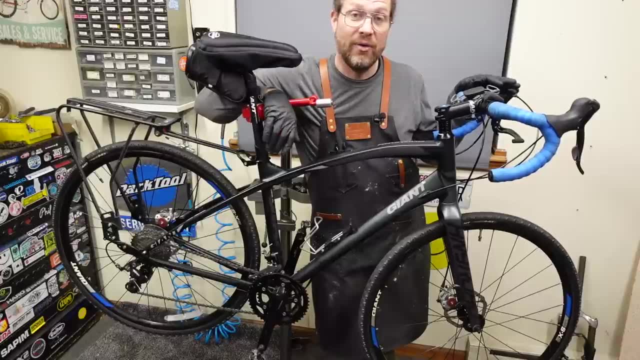 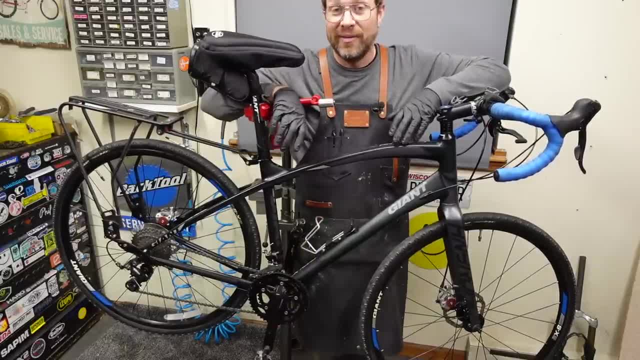 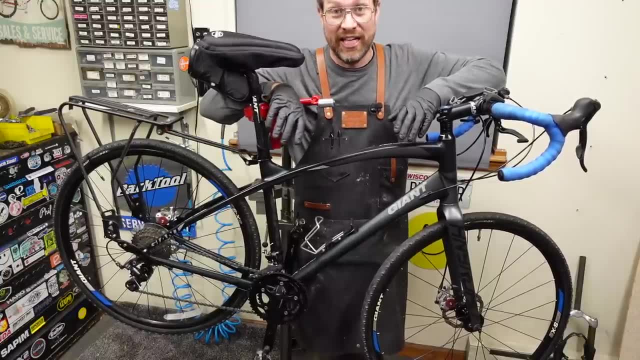 that big of a deal. it's just basic maintenance. I guess what I'm saying is. the main point of this video is: I think this is stuff that anybody can do, and I think it's stuff that everybody should be doing on their own. so thanks so much for tuning in and watching this far. if you made 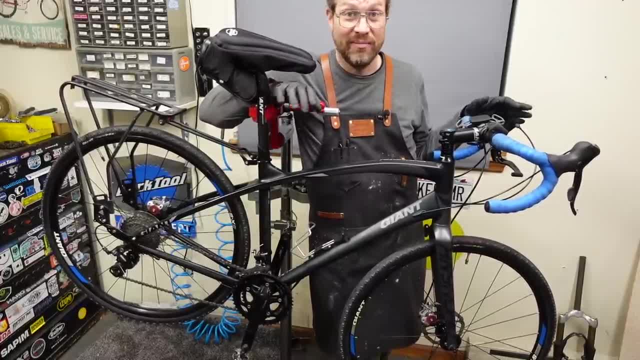 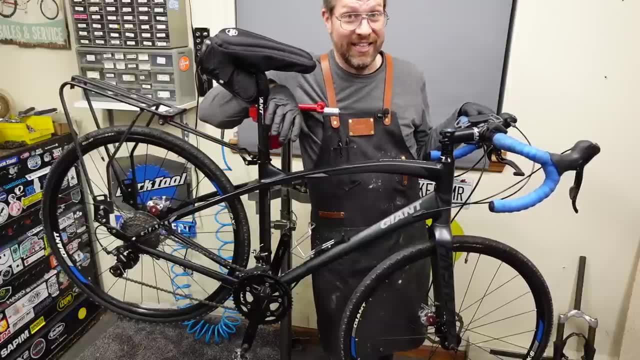 it to the end. you've already supported the channel the best way you possibly can. the algorithm loves that. give it a like. that helps too. subscribe if you haven't. if you really like what you saw, and what I really like to see is a super thing, send me a few bucks, buy me a taco. I love it if you. 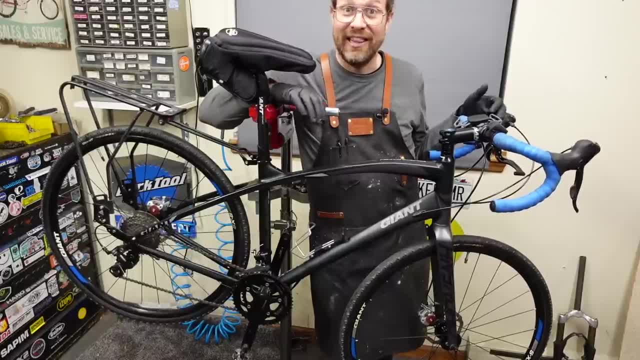 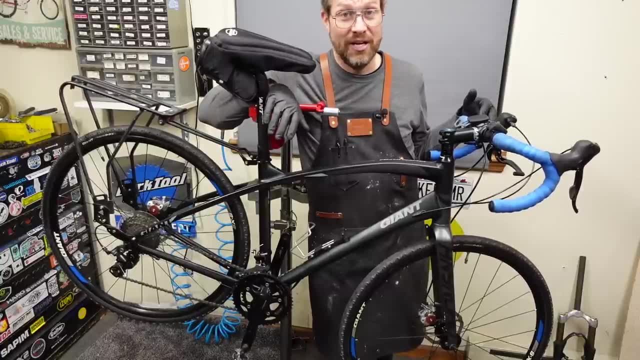 watch some of the other videos and, like those, consider being a member. you get a lot of questions in the comments. I'm just skipping over them now. I don't have time to answer all of them. but if you become a member, give me a few bucks a month. I'll definitely answer your questions for you. 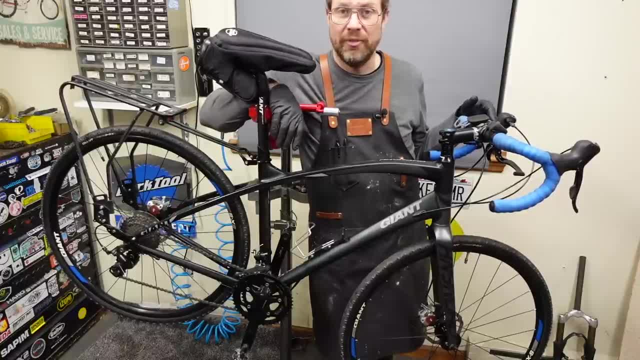 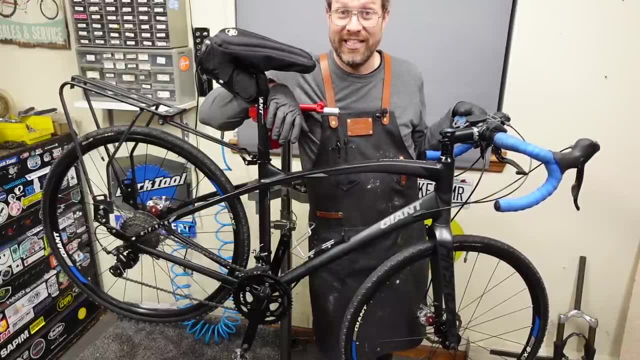 there's other perks too. if you spend a little bit more kind of building out the membership thing as we build a community together, that'll get better over time. the best thing you can do for yourself, though, is click that notification Bell so you and your bike can stay tuned.